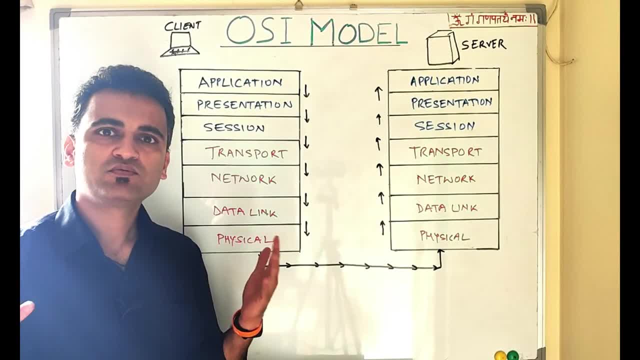 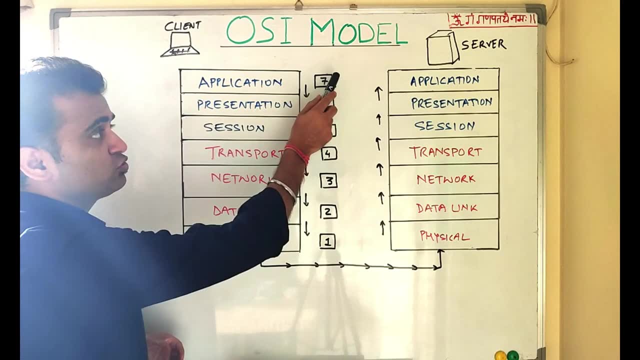 OSI has been there since 1976. And it was started to be officially used in 1986.. So, friends, if we go from top to bottom, your seventh layer is your application layer, your sixth layer is presentation, your fifth is session. 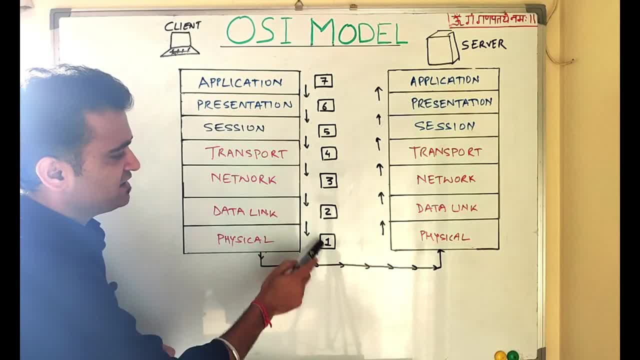 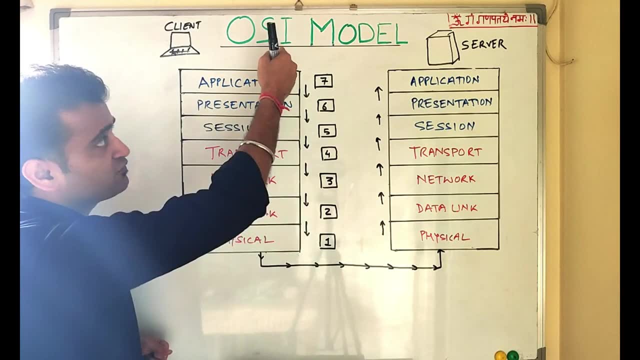 layer. your fourth layer is transport, third is network, second is data link and at the bottom, which is the first layer, is physical And when you are receiving the information. so while sending it it goes from top to bottom, But when you're receiving any information or when you're receiving 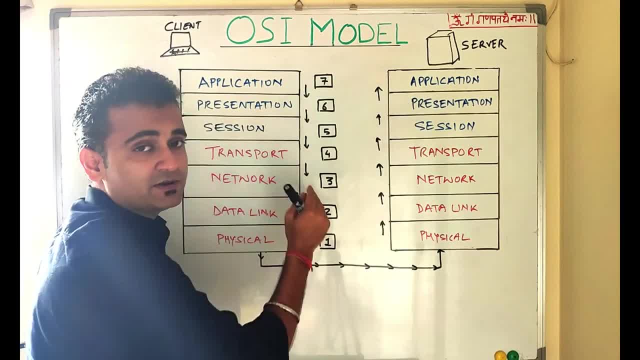 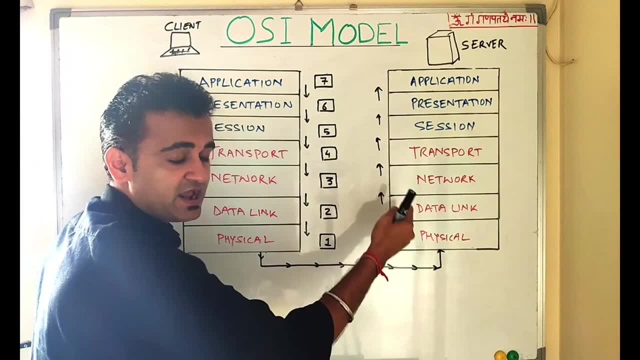 any data packets from the network, then it will go from one to seven. So suppose if a request is sent it will send from application layer down to the physical layer. When the application, any information is received, then it will be received at the first layer and 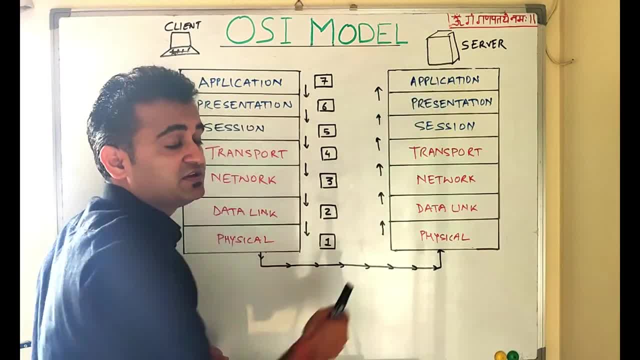 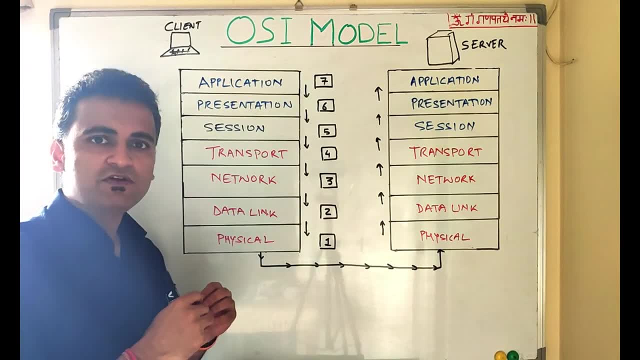 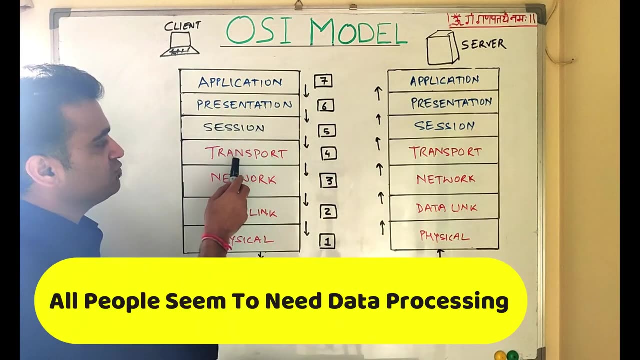 will go right up to till the seventh layer and will be received by the destination environment. So this is a very basic understanding And obviously you would find various ways to remember these layers theoretically. So one very common is: all people seem to need data processing. That is a very common. 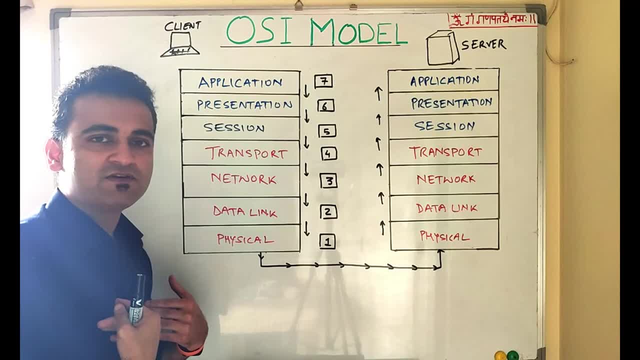 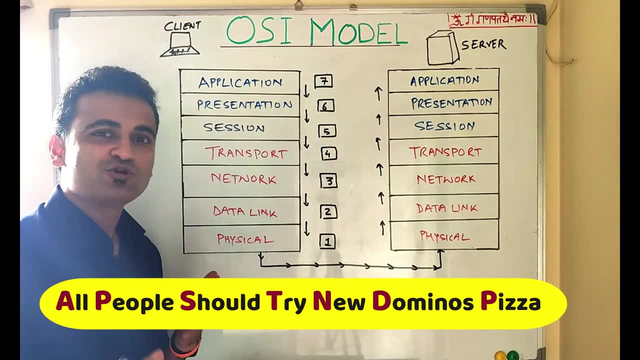 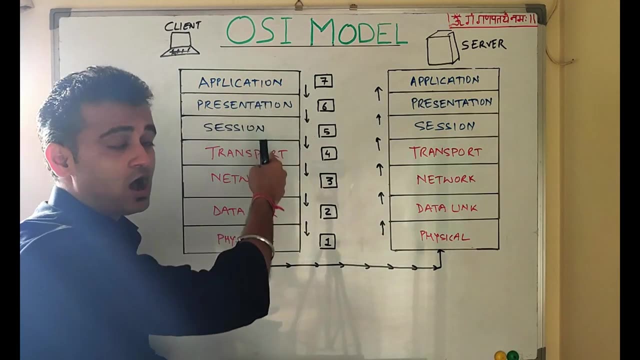 way to learn this particular flow, But I have created my own right now, which is: all people should try new Domino's pizza. So this is more intuitive for me: all people should try new Domino's pizza. So, friends, in order to understand how each and every 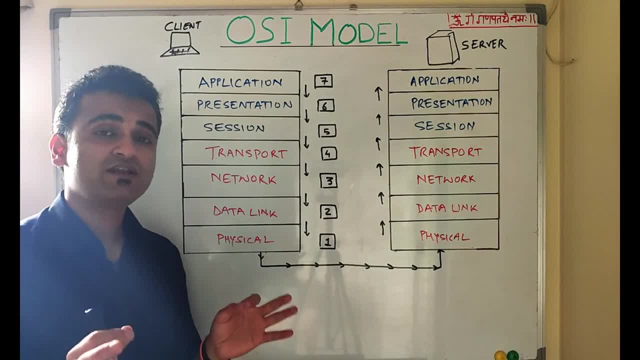 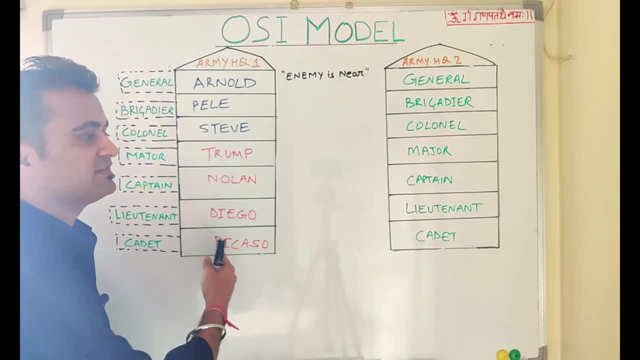 layer works and interact with each other. we will now take a very real life example which will help us understand that, and then we will come back to this discussion. So, friends, consider that these are two army headquarters with seven floors and every floor is being taken care by the respective ranks of these army officers. So at the seventh floor, we have the 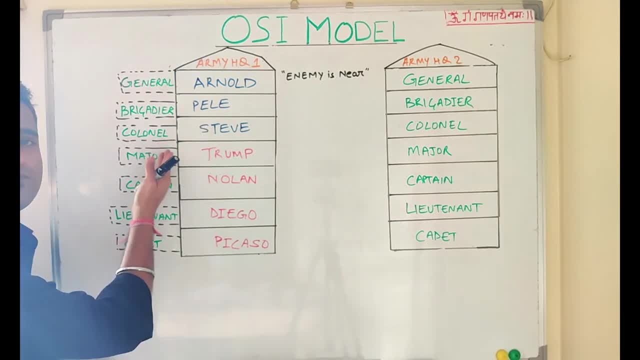 general. at the sixth floor we have the brigadier, At the fifth floor we have the colonel. At the fourth floor we have major. At the third floor we have the captain, At the second floor we have the lieutenant, And at the first floor we have the cadet. So now, similarly, we have another army. 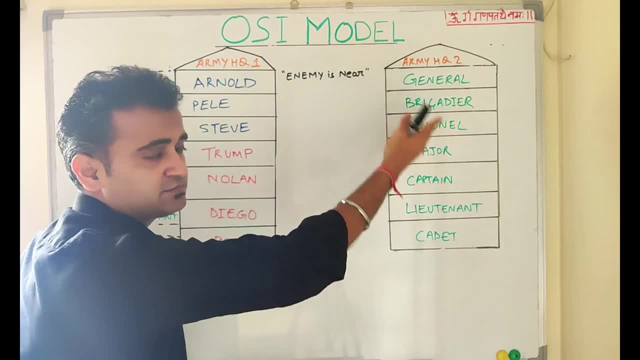 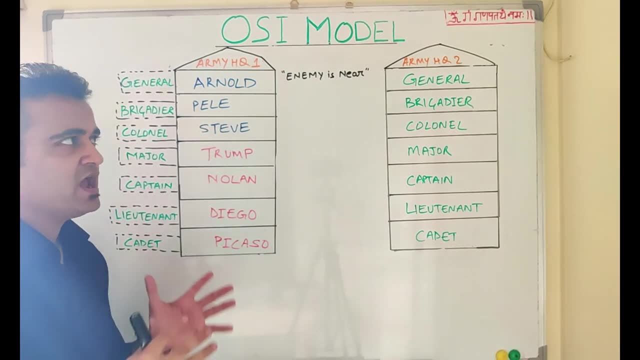 headquarter where we have these ranks Staying in this particular building, in seventh floor building, based on their rank. Now suppose there is a warlike situation going on And this, these two headquarters, are surrounded by enemy and General Arnold gets an intelligence input that the enemy is near and the attack could be at any time, But he could not directly. 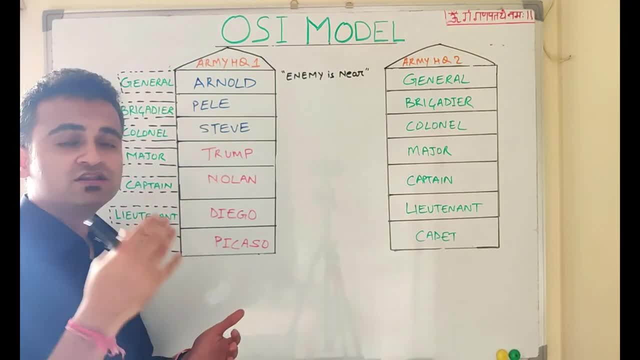 reach to the other general because there is a protocol the way you communicate these secret messages. So that's why he writes a simple note- Enemy is near- and passes it on to Brigadier Pele. Brigadier Pele takes this particular message and understands what he has to do at his level. He has to encrypt this particular message in a way that 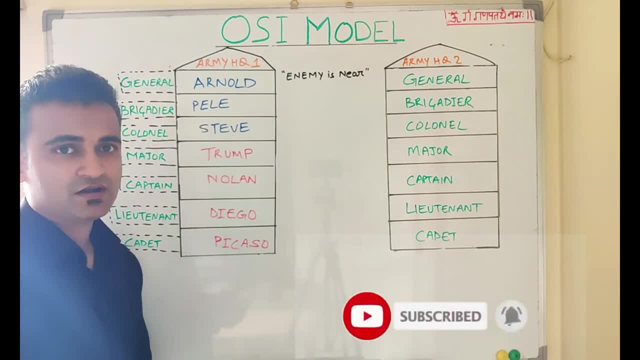 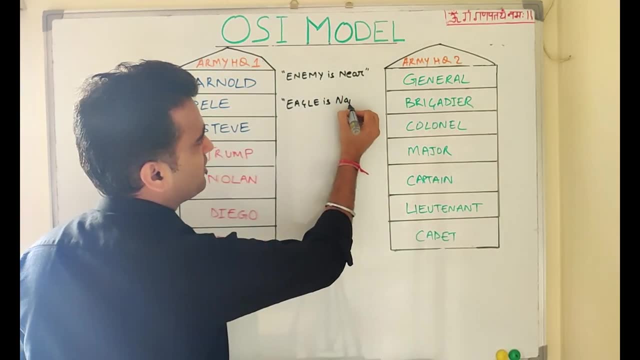 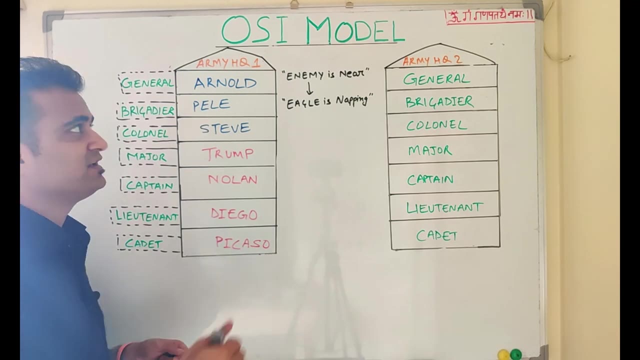 even if it goes into a false hand, it is not recognized. So he changes this message and makes it Eagle is napping. Brigadier Pele takes the message from General Arnold and changes it from enemy is near to Eagle is napping. And this encrypted message he passes on to Colonel Steve. and now Colonel Steve, responsibility is to open a link of 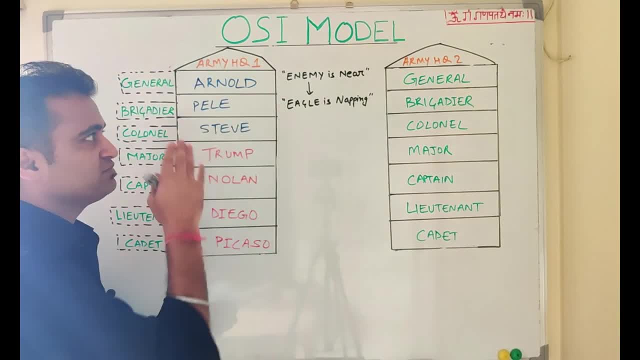 communication with the other building so that this message could go through, because this particular building won't open its gate unless that communication is set up. So what wouldıyor further answer this, asking Colonel Steve to describe a link to you with other building so that this message could go through andpoon its gate unless that communication is set up. So what would Parlament? Ayalla b PowerPoint can navigate Fire jobs or any other bills for any department, But you know it's up to you to decide where tos and pants th. you know. 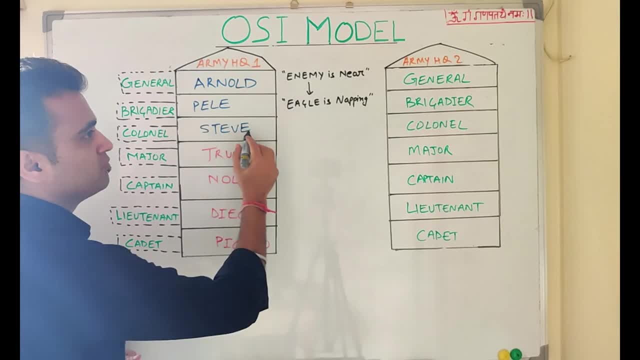 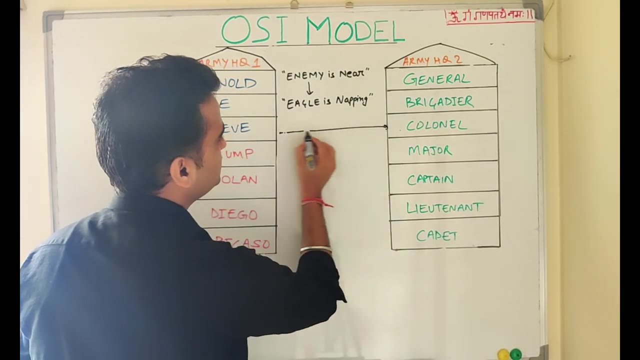 what mr uh colonel steve would do would call the colonel sitting on the fifth floor of the other building, give a passcode, a secret code, to exactly identify that he himself is calling, and then this particular link, a communication channel, will be open between these two uh kernels and there will 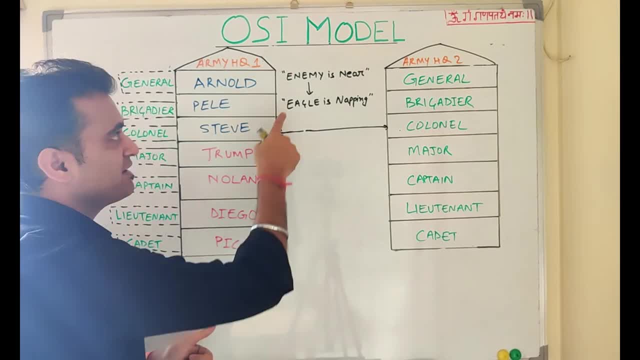 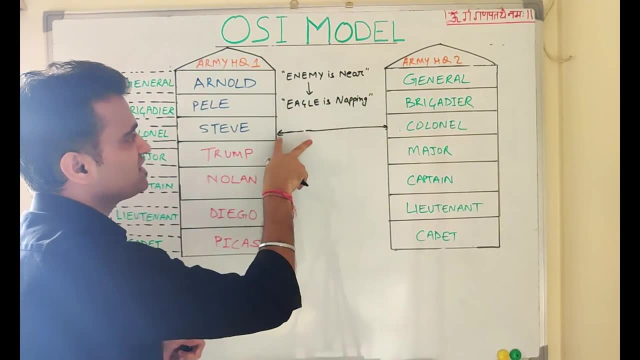 be a phone line, open a walkie talkie to be open till the time this message, because we have very limited time to reach this message to the general in the other building. that's why, till the time these two are on the phone, this message would continue to go through to reach, uh, the correct uh. 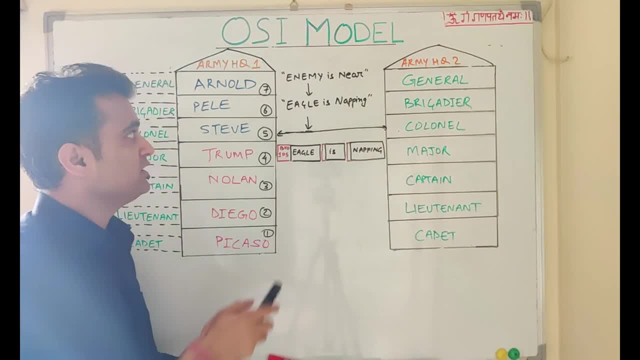 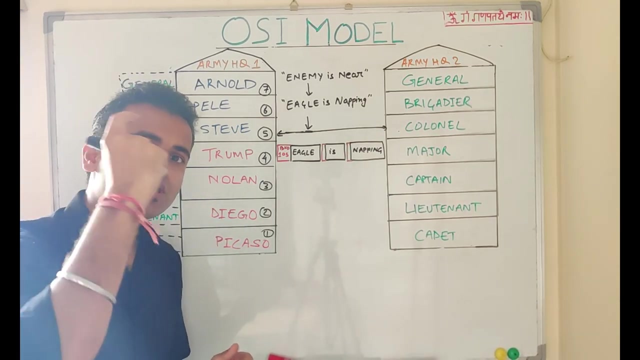 destination. so once this particular communication link is open, uh, colonel steve passes on this message further below to major trump. now major trump divides this message to multiple small, small segments, and this is to ensure that the message reaches safely to the other side, and that's why he also adds one particular additional. 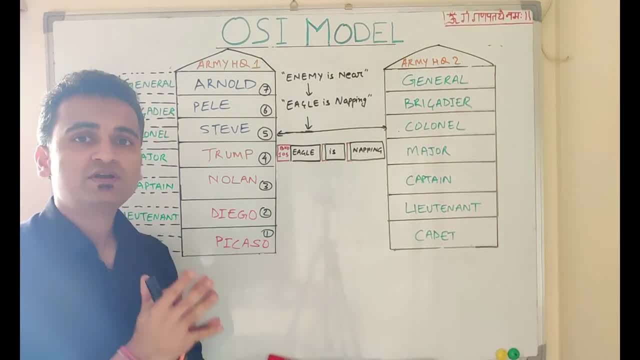 information in this particular segment, which is the building number, because without knowing the building number, this particular message might get lost. so, in order to further secure and further make it efficient, he breaks it into three different segments, which is Eagle is napping and it adds, he adds building number 105 in front of these segments and then he 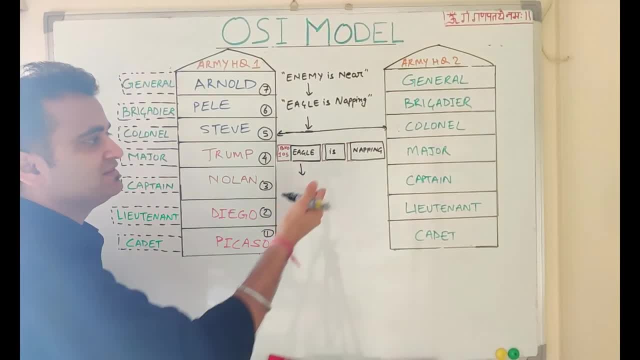 passes on one segment below to the third layer, while these two segments wait for their queue. so this particular segment is now going below to Captain Nolan. Captain Nolan's responsibility is to further ensure to guide this particular packet on a specific route, because from this building to this building. 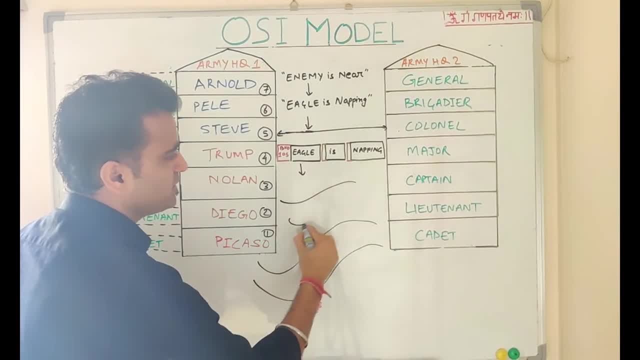 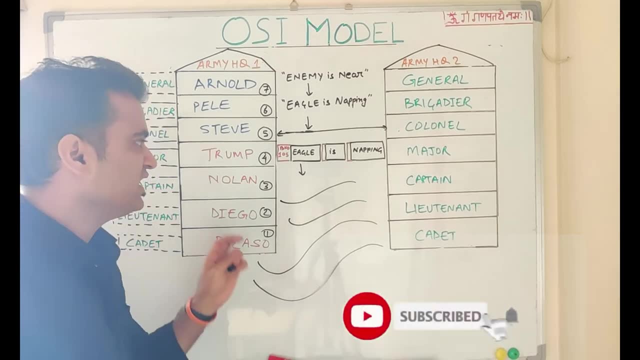 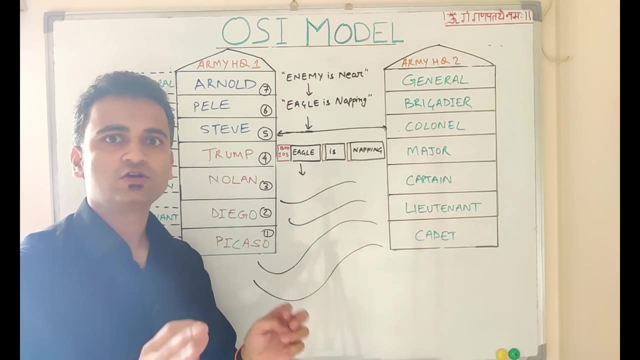 there are multiple routes. okay, so there could be multiple routes going from this building to that building, but Christopher Nolan's responsibility is to make sure that it assigns a very, very clear route to ensure that the message reaches safely, securely and at a very fast pace. so that's why Christopher Nolan adds the routing details, the route, the road with which this 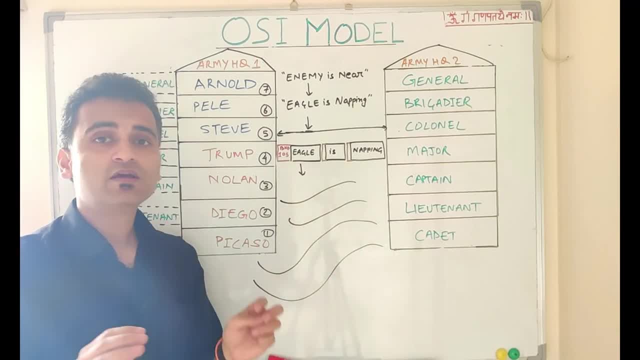 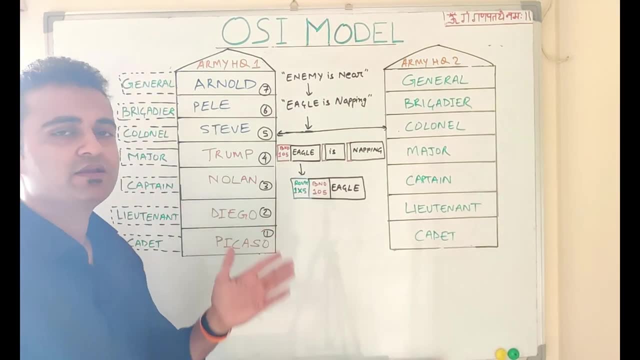 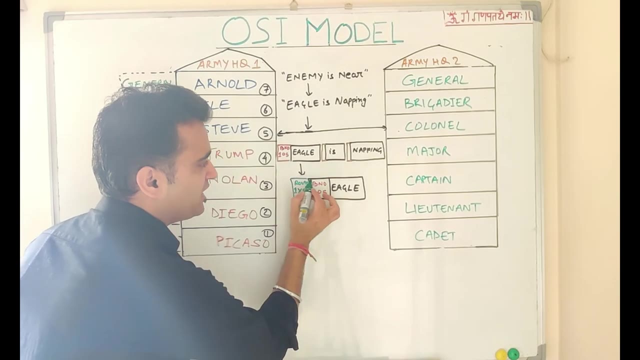 particular building, from this particular building to this particular building, that particular route to take would be added in this particular packet. so let me show you so now. Captain Nolan has added one additional information in this particular segment. so now what it has done is it has added routing detail, and now this particular 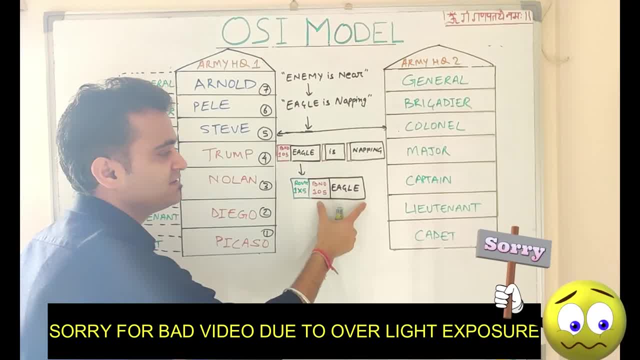 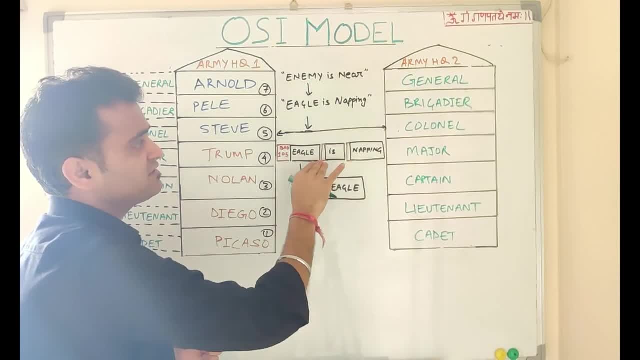 route only will be selected. Route 1XY would be selected while sending this particular information. so just remember the flow till check. here we have the information. after this, these three layers here, this information was changed into this particular information, or my rough Fluff. it is just a little looping of numbers and theze three of these three. 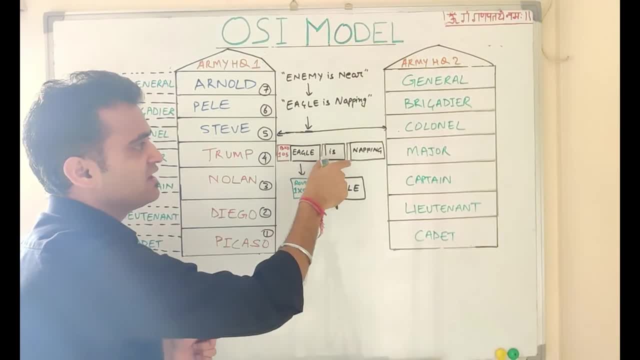 mandatory routes are now recorded and can be done so. if you always have one, Add in Selected multiple small segments. after that this particular segment was further broken down and added routing details. now this particular segment has now become the packet, so once we have the route details further, captain Nolan sends this. 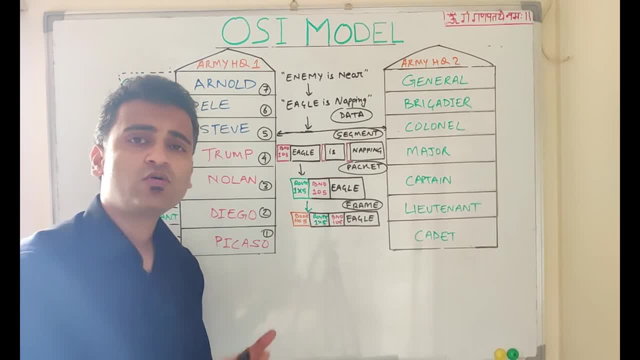 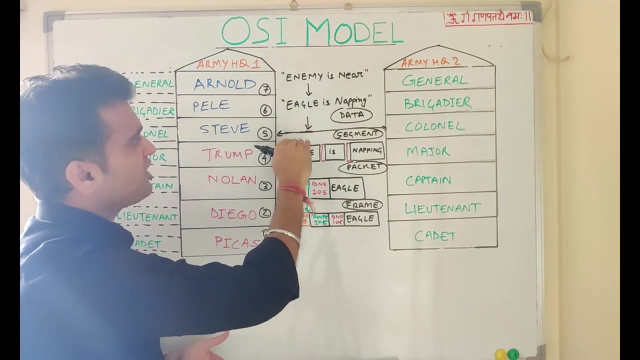 information to left in and Diego, and left in and Diego adds the door number, the door behind which this information has to go through, and that door number is door number five. so now you can see that this message started as a pure information or pure data, and after layer 5, after colonel Steve established, 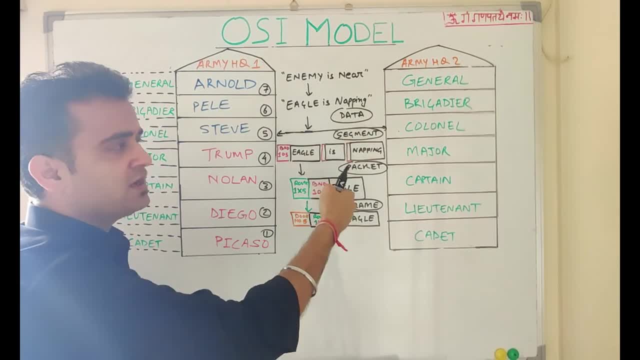 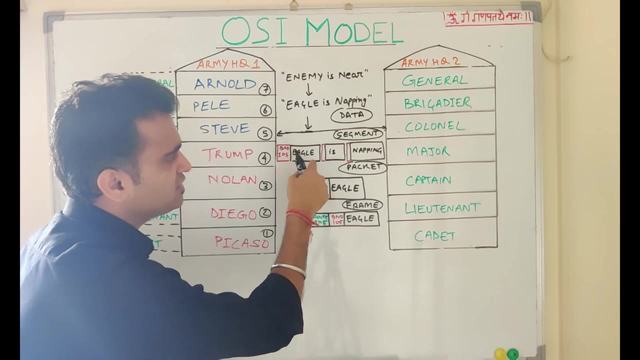 that communication with the other colonel. this then started breaking into segments. major Trump divided it into segments, then captain Nuland further divided it into packets and then left in and Diego further divided it into frames. so now you can see that this particular Eagle information is now flowing below. 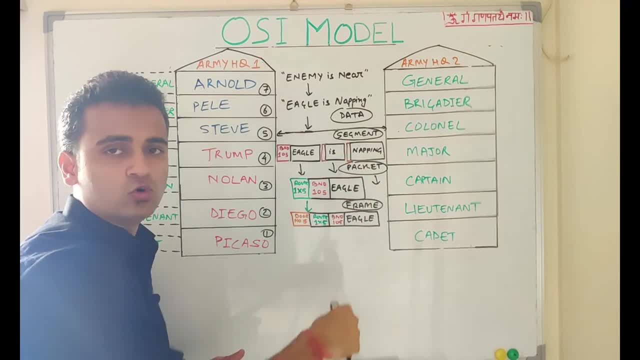 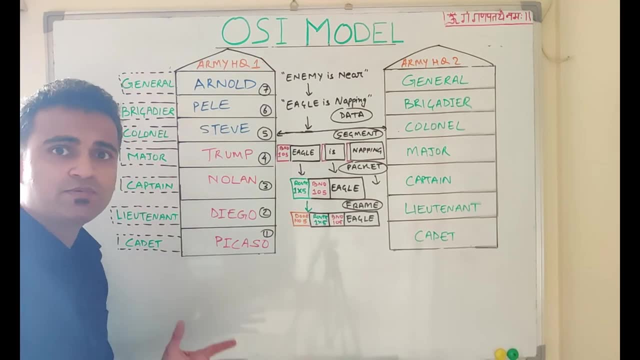 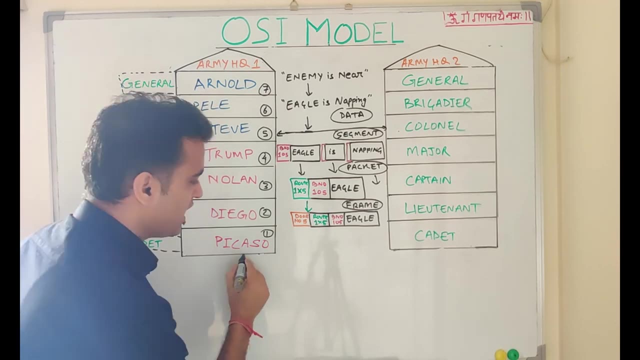 but parallelly these informations will also follow. so ultimately, once this whole setup is done, the last level is of cadet Picasso. cadet Picasso is actually the ground worker, the field worker who will take that risk of taking that information, running through and making sure he hands. 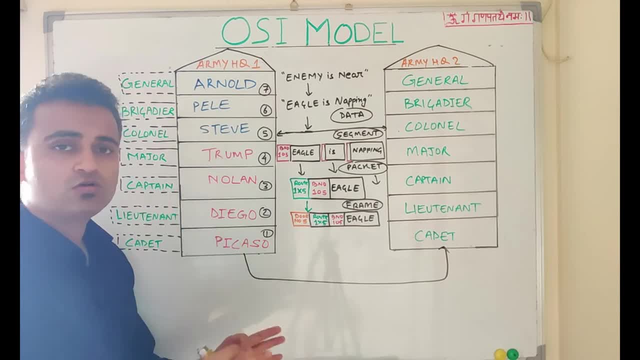 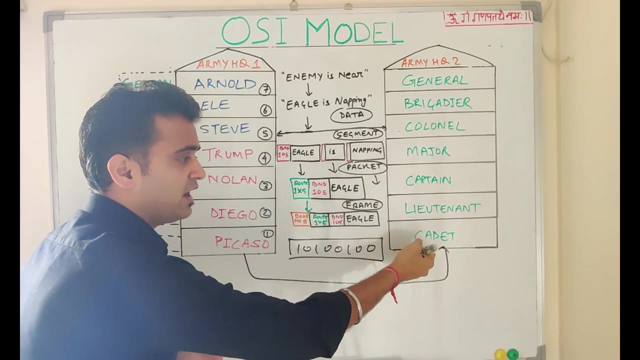 it over to this particular cadet here and that particular information will be converted. this whole piece of conversation, piece of information, will then be converted into binary numbers. so these binary numbers would be then be decoded at the cadet, at the cadet level of the other resource. so 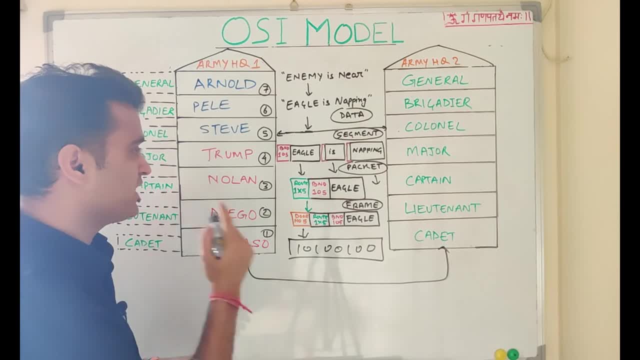 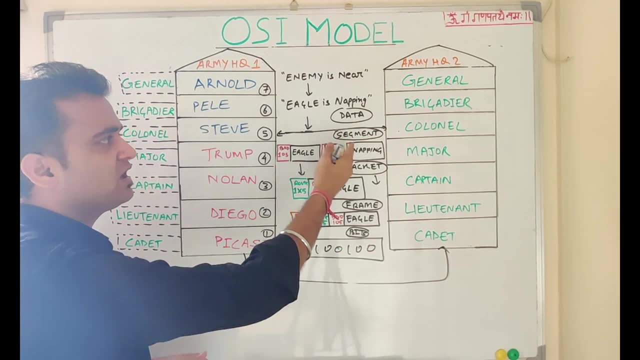 you can understand that. now, what has Mr cadet Picasso what has has done? is that he has further changed this particular information into bits. so now you have data, data then converted into segment, segment converted into packet, packet converted into frame, and then that particular frame was: 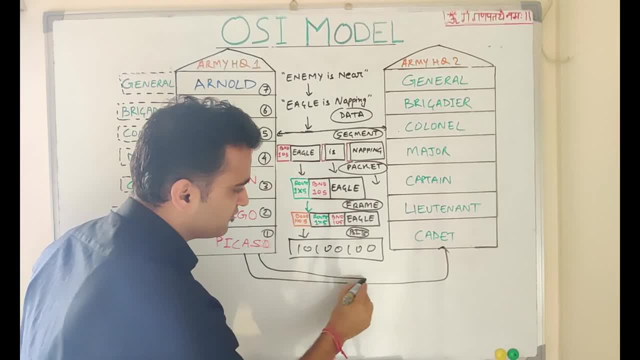 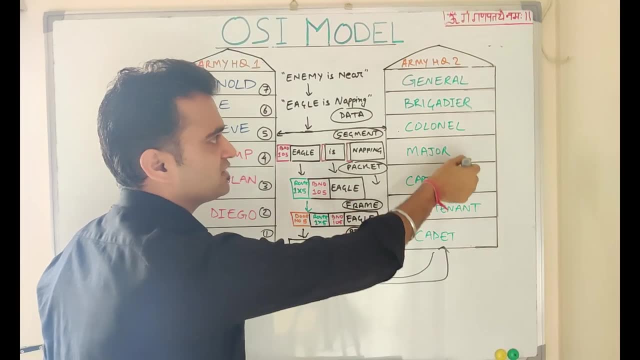 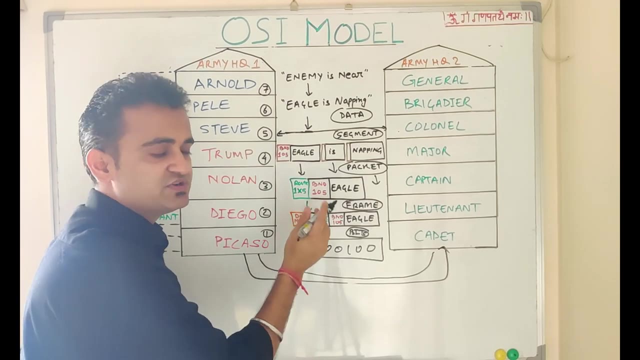 converted into bit and then the actual cadet took that information and center, handed over it to cadet on the other side and then this particular cadet further made sure that this information goes up and all these layers and all this you know additional headers which are added to this message gets cancelled. 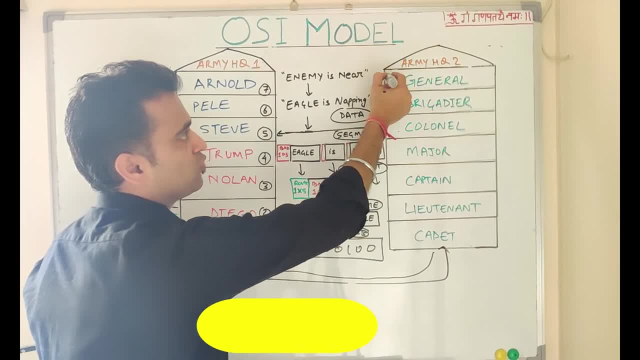 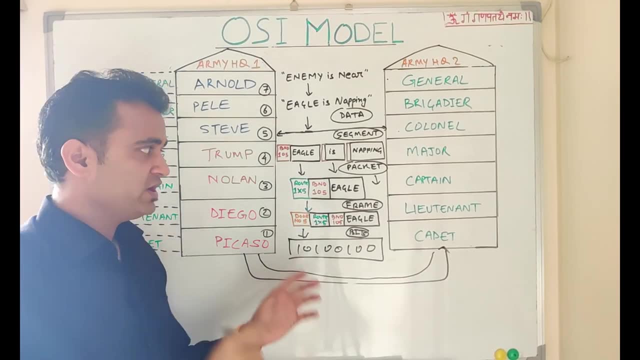 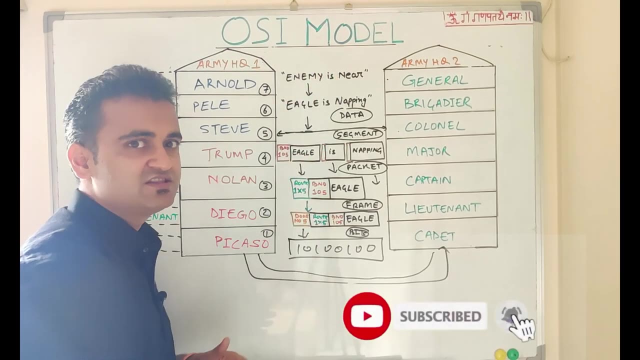 out, cancelled out, and then the real information goes to the general, and general tells understands that, yes, the enemy is near and he should be ready. so in this particular whole flow, you understood that how information as good as a very simple information like this could be very securely passed on to. 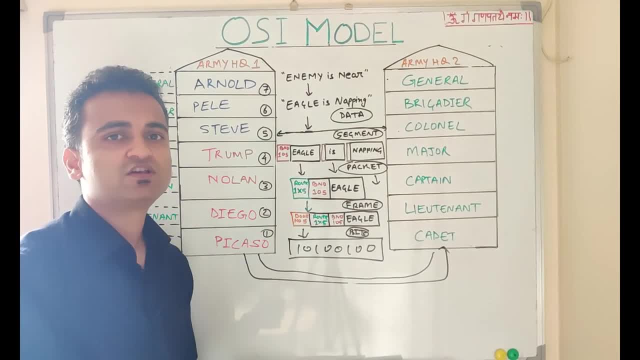 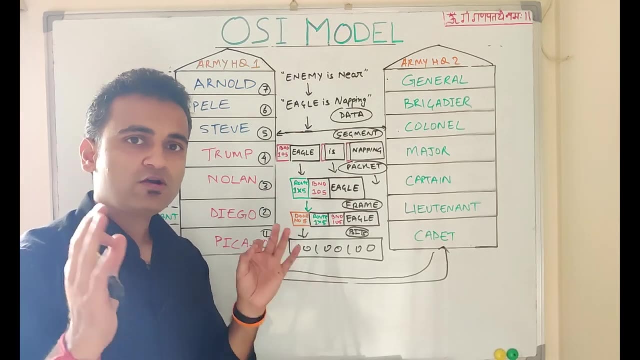 multiple layers and ensure that it reaches on time, safely, securely, to the other general. so now I think you have got an idea, but let now let's go back to our actual discussion and understand how OSI model fits into this whole setup and also the example which I have. 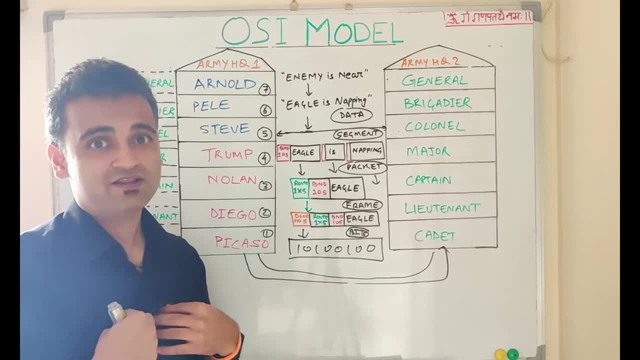 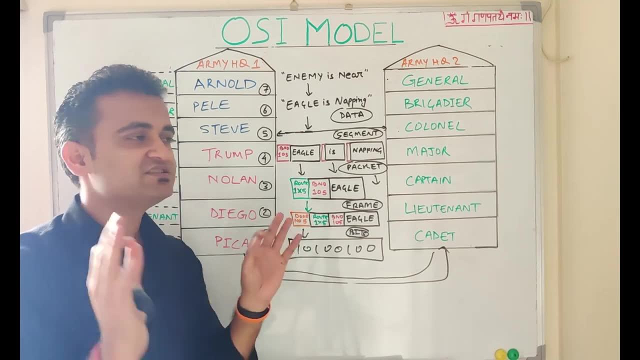 taken is that the OSI model fits into this whole setup and also the example which I have taken, the army, generals and ranks. I have taken it on my own and experience and knowledge don't quote me on that. and also it might sound that some bits are not relatable exactly, but this is just to give you an understanding. so, friends, 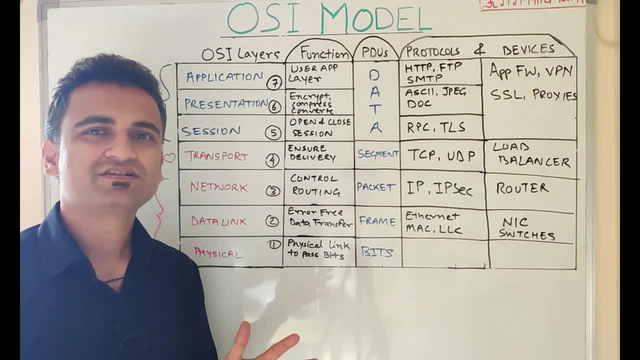 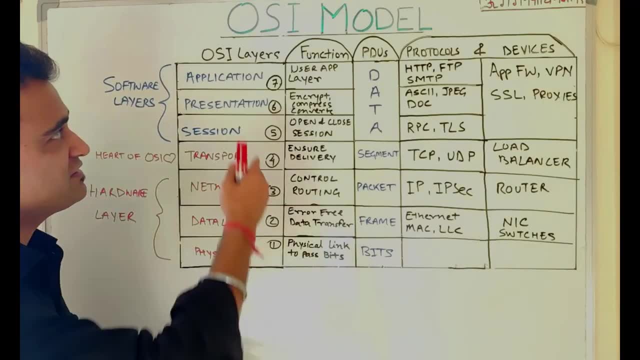 after looking at the real-life example, now is the time to go back to our OSI model and understand a bit of theory. but we'll try to make it interesting. so these are the seven layers which we discussed and, as you can see, I have highlighted three layers in blue. 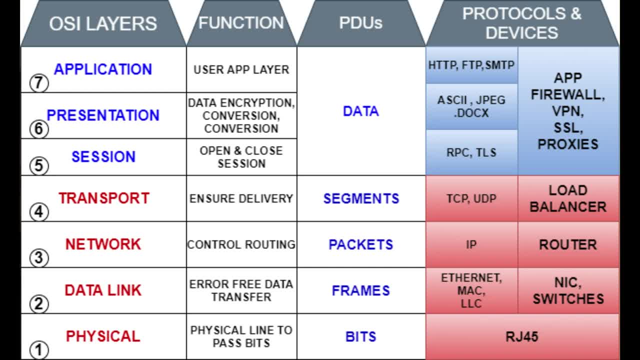 and rest four in red, because these three layers are primarily software layers, where the- which which resides at the software application level, but these are actually the actual hardware layers- and the transport layer sits as an interface between the software and the hardware, and that's what is called as the 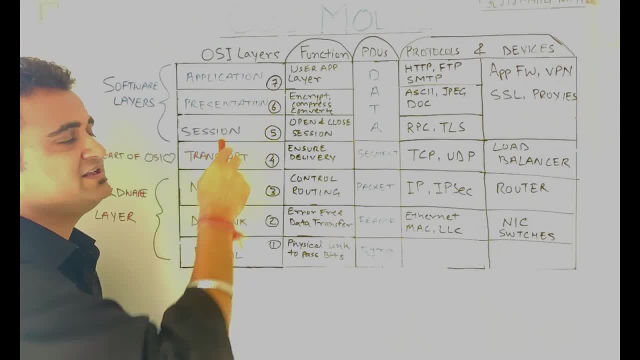 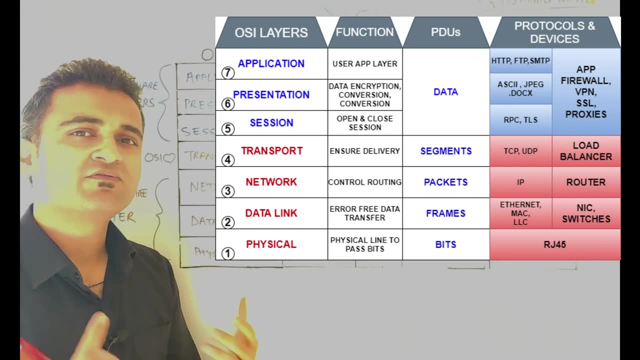 heart of OSI. so now let's understand what exactly each layer does, what kind of data or the protocol, data units, its processes, and then what kind of devices and processes it uses. and then what kind of devices and processes it uses and protocols every layer uses. so, at the application layer, as you can see, this, 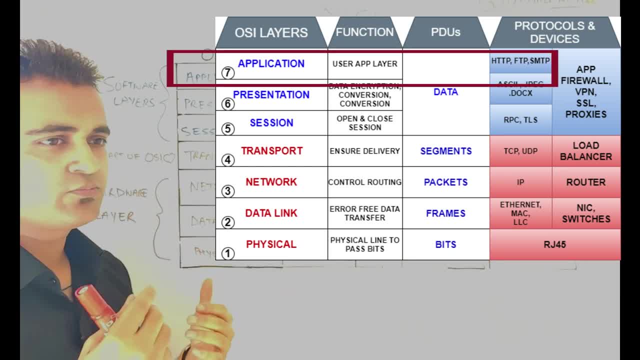 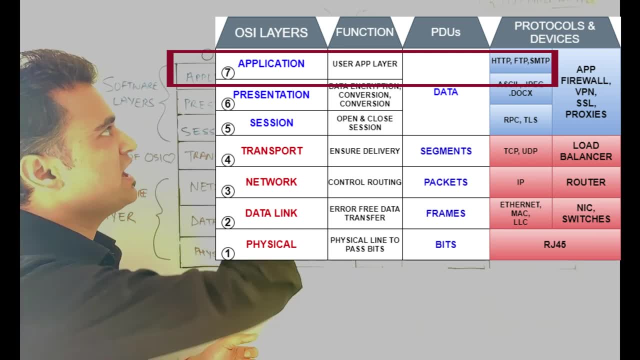 layer sits very close to the end user. so suppose if you are trying to send an email or if you are typing googlecom, then you are actually invoking a network communication at sitting, at the application layer. at this particular layer, the protocols which we use are very famous protocols, some protocols: 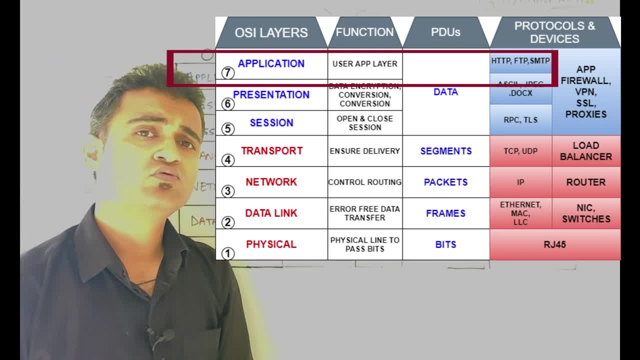 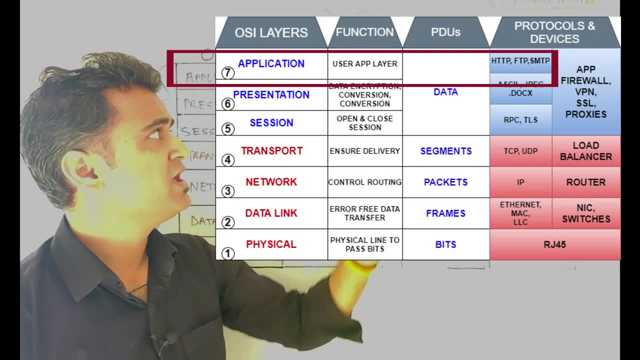 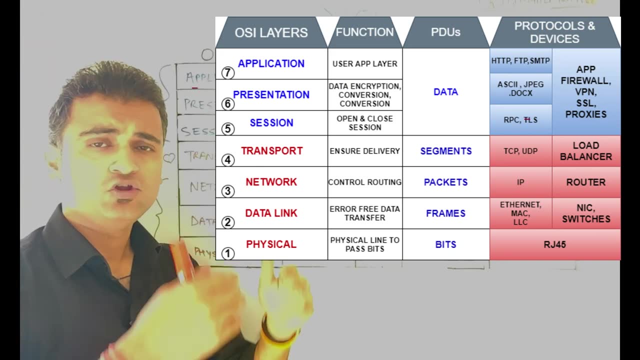 there are many, but some protocols are HTTP when, when you are using, you know we, when you are trying to browse anything over the web, and then you have FTP for file transfer protocol, and then you have SMTP, which is a mailing protocol, and then, at the presentation layer, you when? 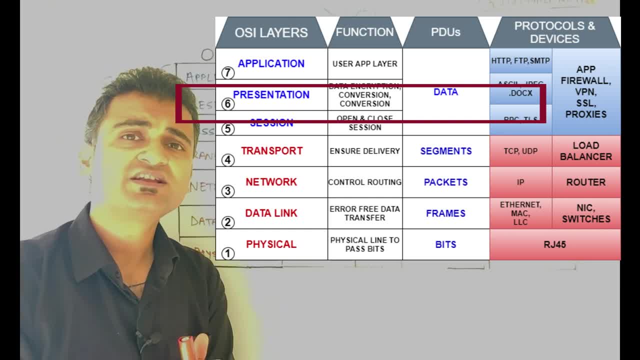 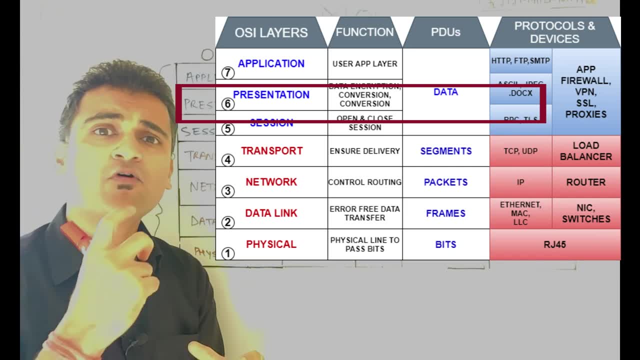 you send the information from application to the presentation layer. the presentation layer actually compresses, encrypts the information, compresses it and makes it in a format which is more understandable. to suppose your data is right now in English but you want to process it in some other language? 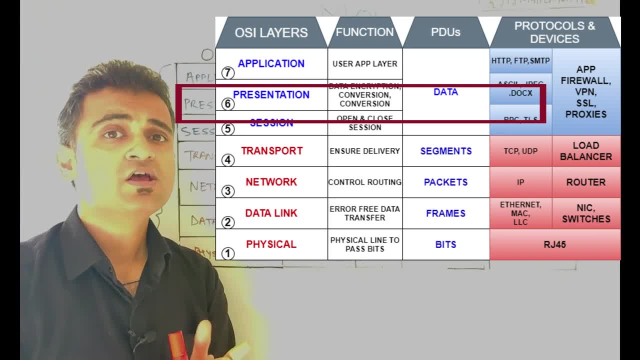 and this particular layer could do that. also in our previous example, when the general wanted to share this information that enemy is near near, this particular you know layer converted that message from enemy is near to eagle is napping so that no one can, you know, look into the exact information. so this particular 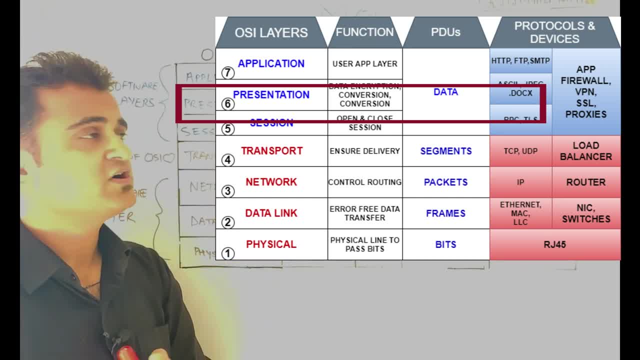 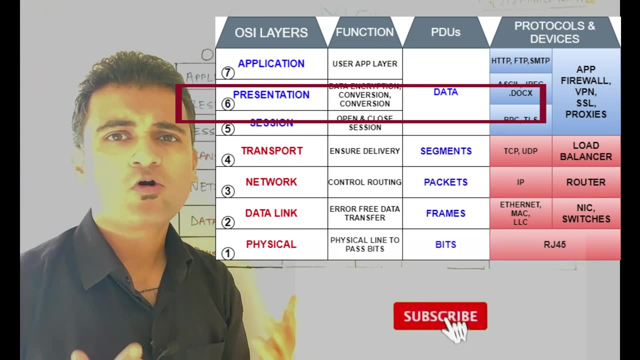 layer, presentation layer, has this particular function of encrypting data compression, data conversion. all those kind of functionalities are done at the presentation layer. some, some major protocols, or you can say, are ASCII, JPEG, doc. so all these kind of formats which you can, you know, convert to, can be used. 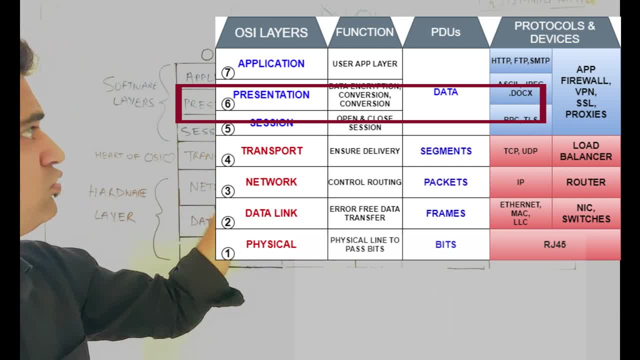 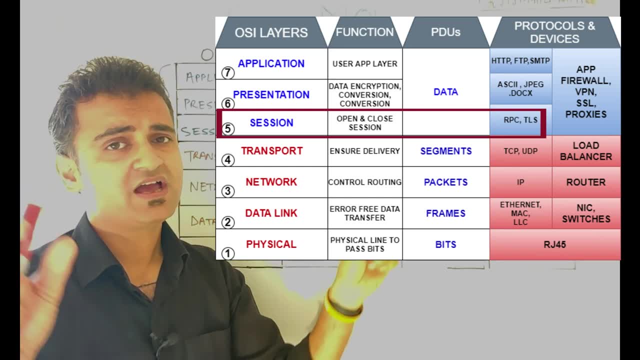 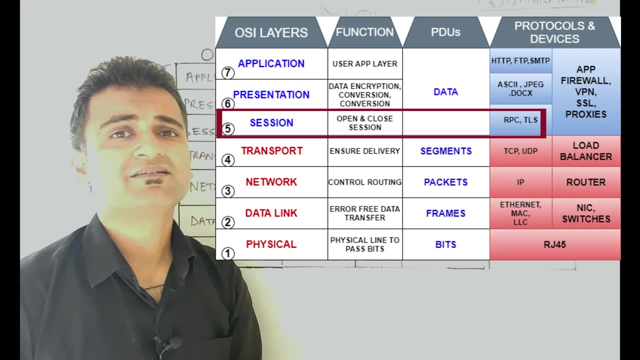 at the as a part of presentation layer. now, going down to the session layer, this is the time when the kernel called the kernel in the other building, gave a passcode and enabled that particular link so that the message could go through. it establishes the session between the sender and the receiver, and. 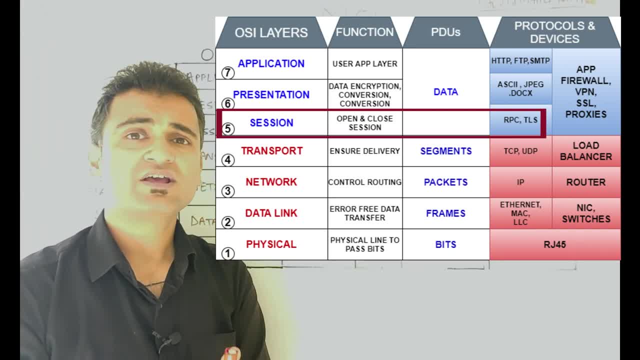 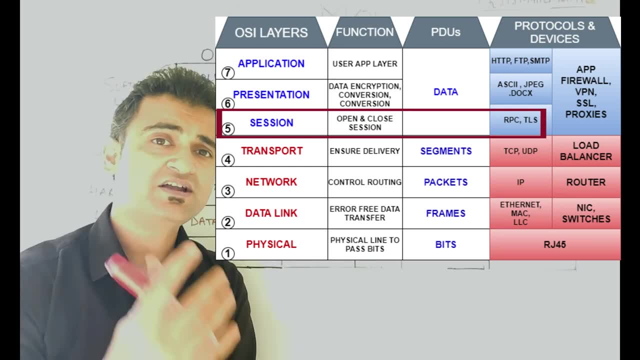 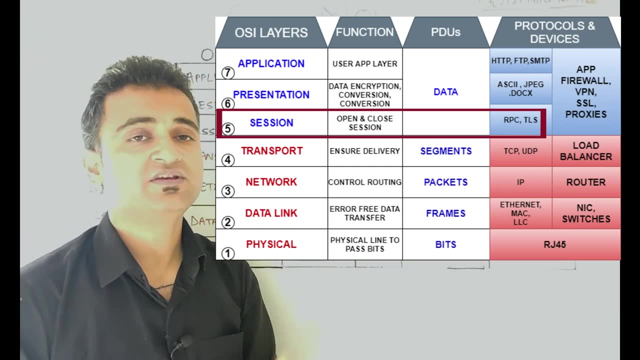 it also makes sure that there is proper authorization of what message is being sent. so even before sending any message there has to be an authentication and authorization to ensure that you know a proper sender is trying to send any data to the receiver. so at the session layer, if you remember, the kernel called the 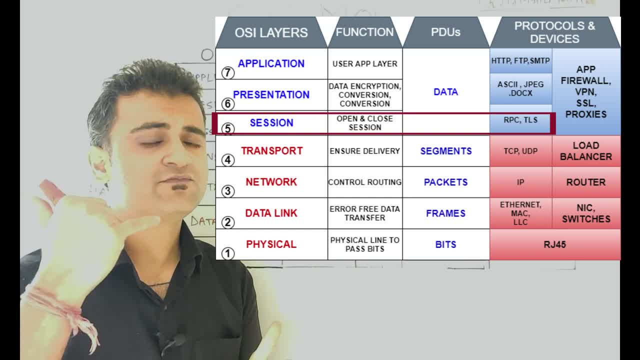 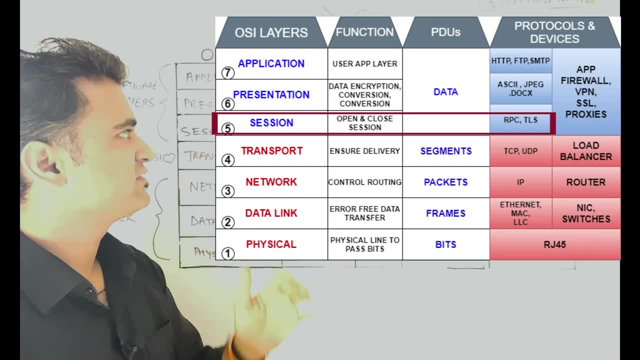 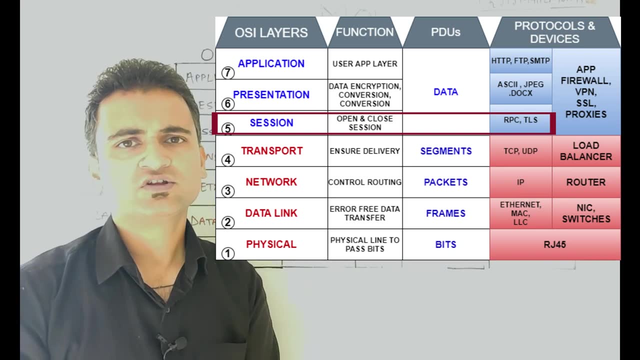 other kernel in the building, gave a passcode and opened a telephone or a walkie-talkie link so that the message could could reach to the other building. that is the function of a session layer. it opens and establishes a connection, a session, and then, once the whole network communication is over, that particular 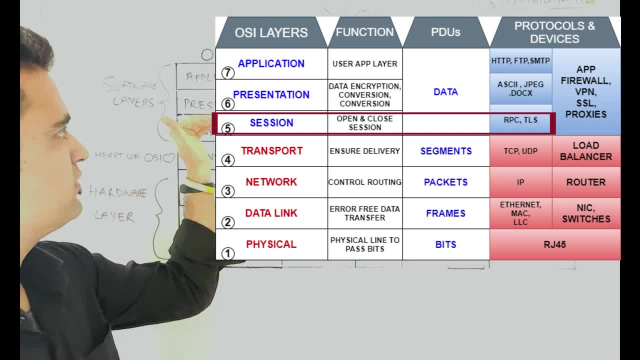 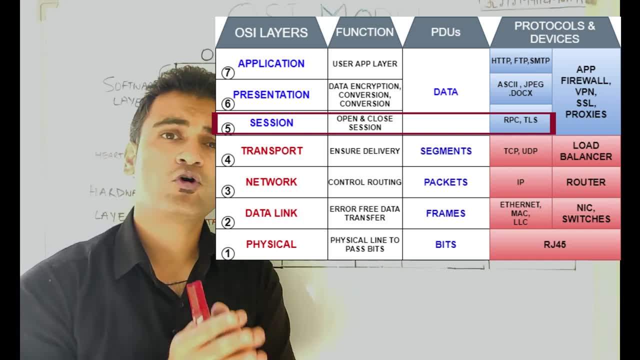 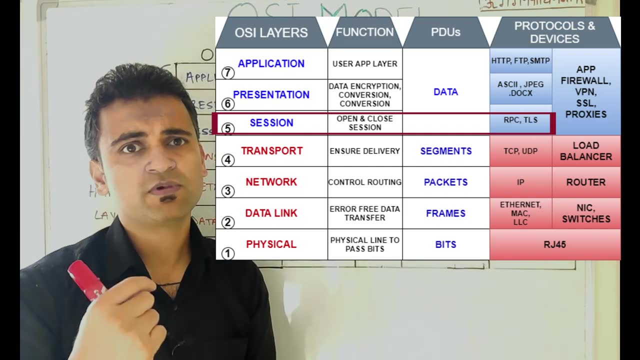 session is, you know, closed. so this particular session layer uses protocols like TLS and RPC and in this particular session layer we also have authorization and authentication. you remember we gave a secret passcode to the other kernel so that he could establish that this is coming from the right source, that that. 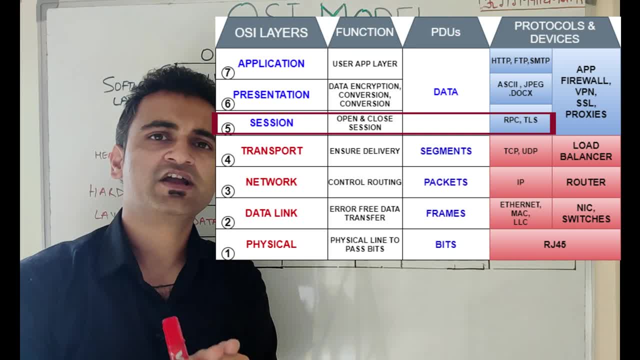 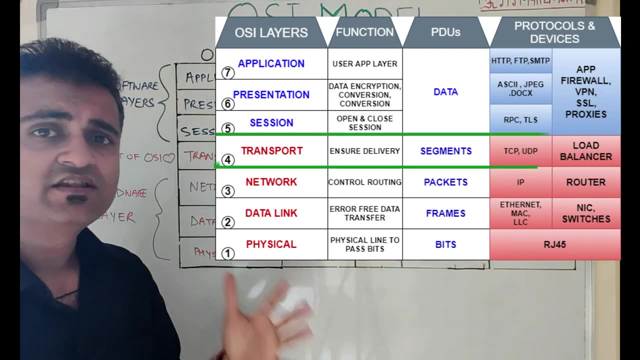 you know, this is going to be the right location in this particular session layer. so all of that. the process of authentication is often different and it is first of all necessary to know that which is the error, which is the source of information, and then, after that, you have to identify this error. so your 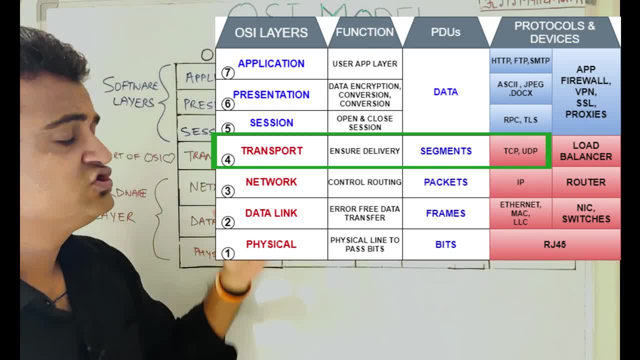 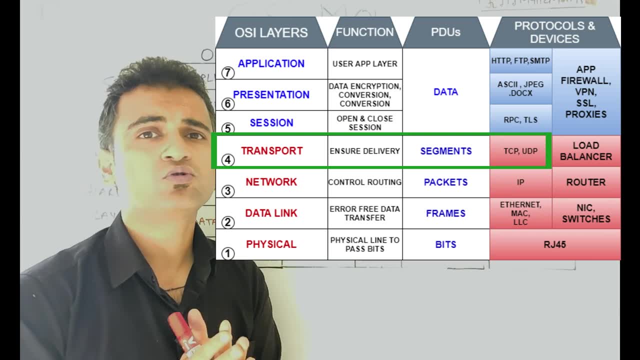 processing, is this error, is your data, and then you have to identify this error and then, after that, you have to identify the error, and then you have to identify the novel error, which is something called the error of the error, so that if you are removing an error and you have to connection it to the wrong place, then you 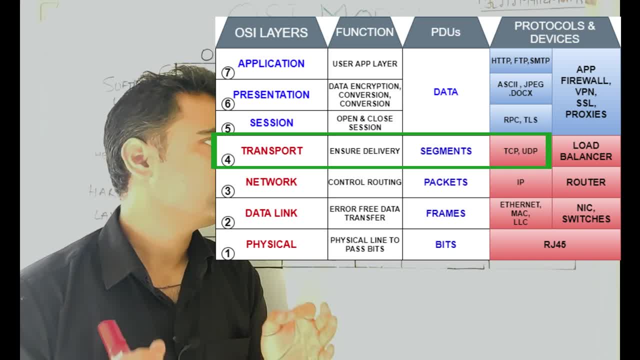 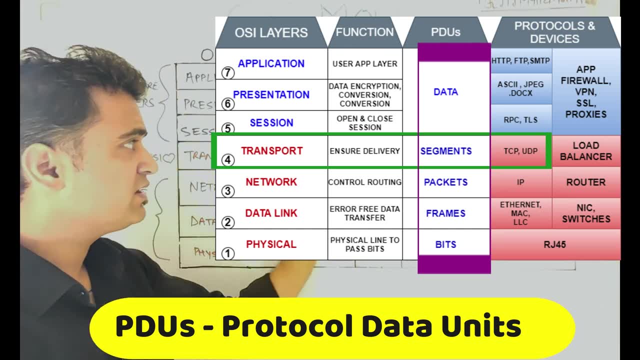 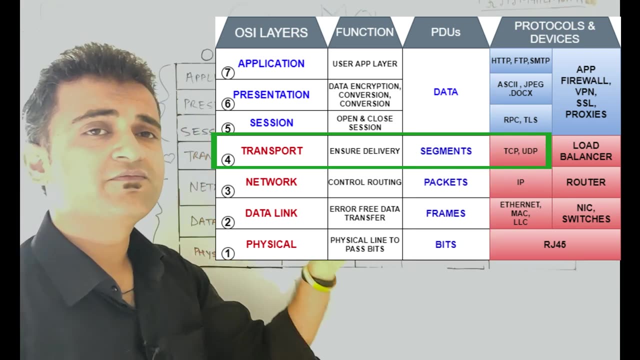 TCP protocol, the transportation protocol, is used to take the data. So one more thing: we have not touched the PDUs. we will come to PDUs, but understand this: that whenever we have to ensure the delivery of a message, transport layer plays a very 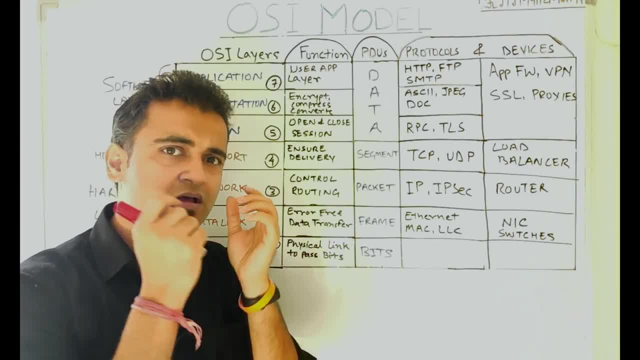 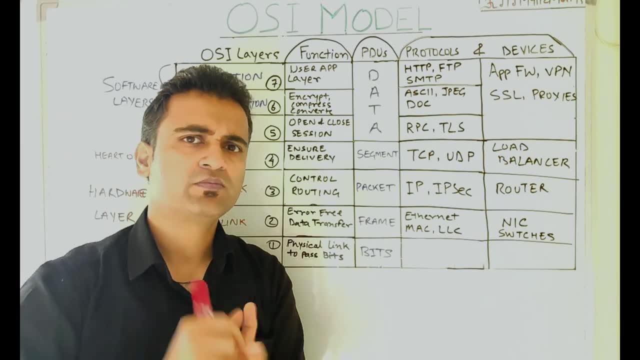 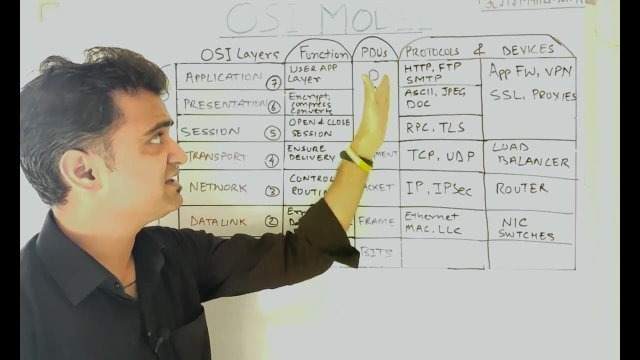 important role because it actually adds the poor details, for example, to the particular message. So let's suppose if you are trying to hit a Tomcat server, suppose, so what is the default Tomcat port? It is 8080.. So then when you are sending this data till here, this is pure data till here. this is. 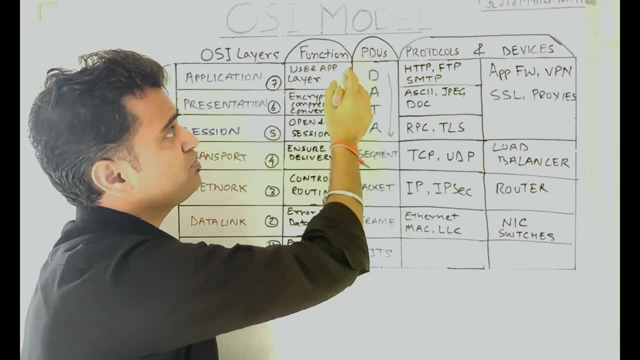 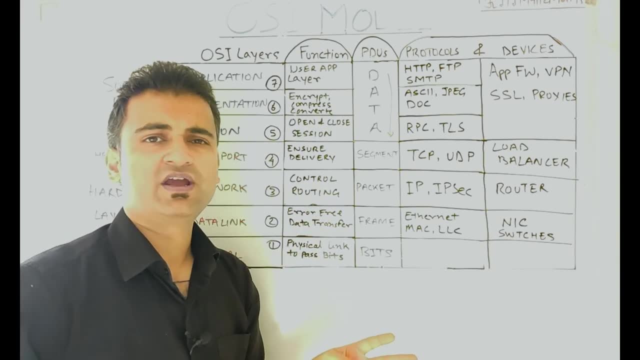 pure data. After that, this starts converting into PDUs, which is called as protocol data units. What are protocol data units? This is the way we distribute the data in order to make it flow into the network communication. So what we do. 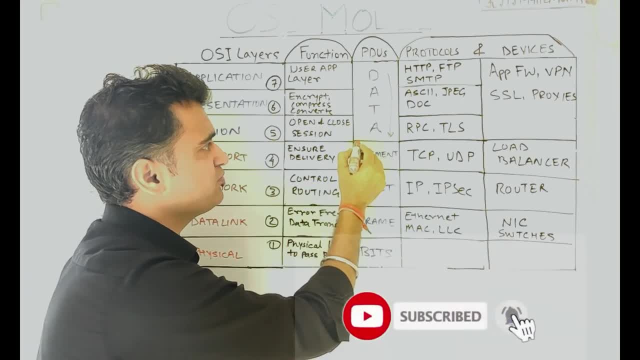 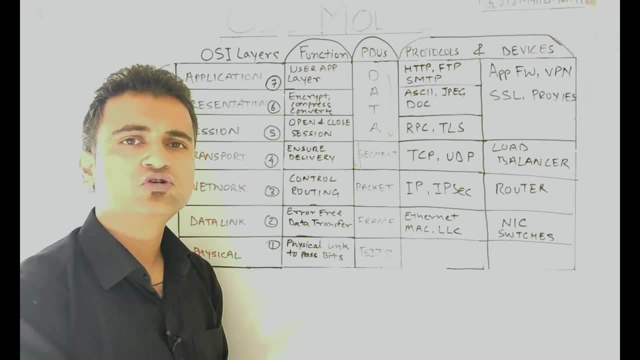 We take this data and add a Tomcat server, A transport header. a transport header is added in front, And what kind of transport header we could add? We could add the port details. So suppose you are trying to reach a web server, then the default port could be 80 or 8080 or 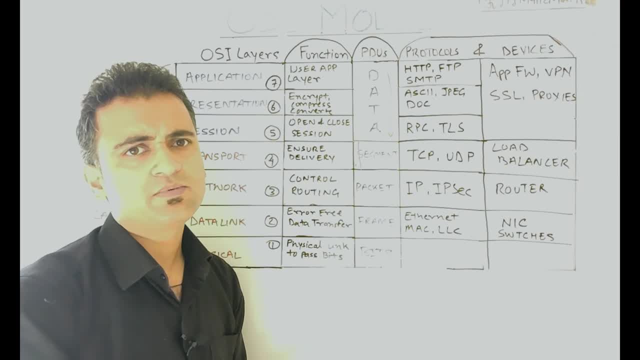 whatever. Suppose you are trying to reach a database, then there could be a database port for enabling that particular communication. So in all that TCP protocol is used. But what is UDP? UDP is also another protocol, user data game protocol. So what is UDP? 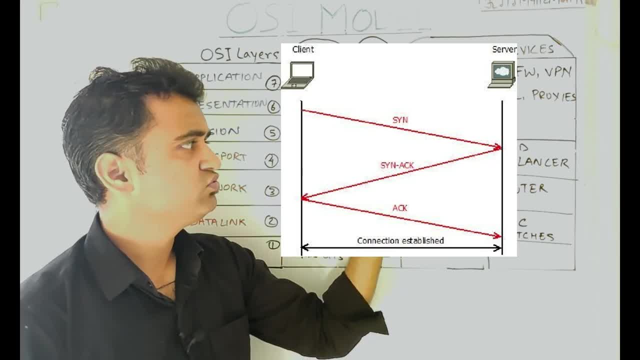 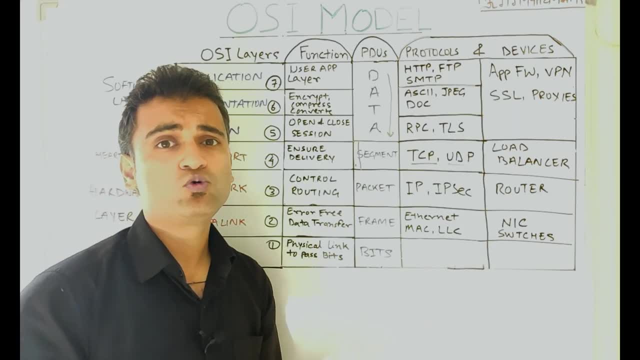 So how? TCP and UDP are different from each other, So TCP uses three-way handshake shape. But what about real-time data transfer, where the data volume is huge? You do not have enough time to have a three-way handshake, So user datagram protocol just sends the message and does not wait for the acknowledgement. 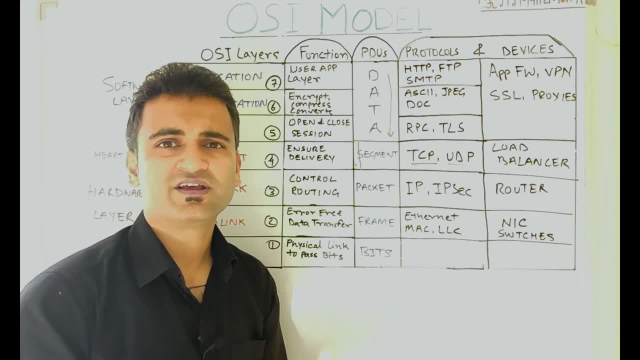 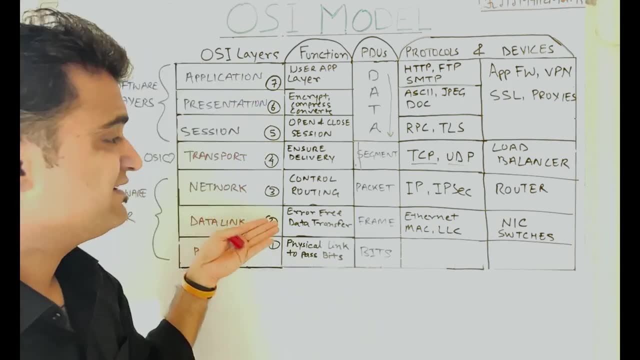 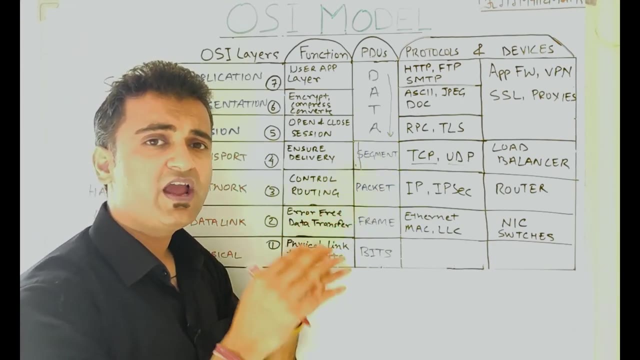 So suppose for real-time video processing or voice processing systems UDP is used. Suppose you are streaming a movie in real time, then that might be coming from a UDP protocol. But what about network layer? This is the layer where we break this segment further and we add further information and 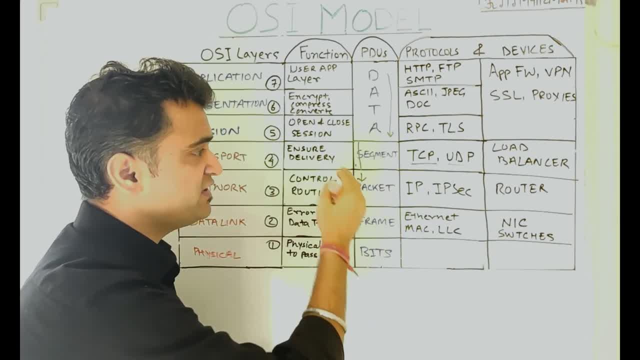 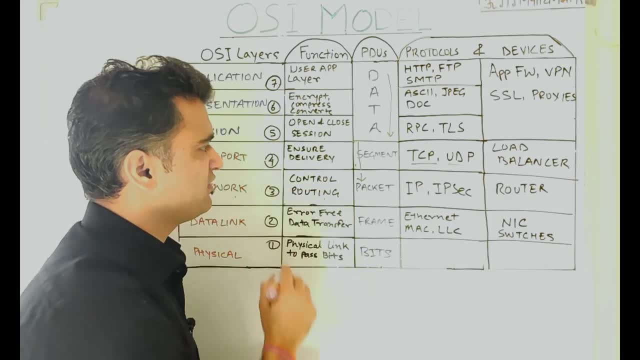 make it a packet. So this segment goes down and we add one more header- information- in this, which is a network header And what can be the network header In this particular layer. you decide the routing- how you want to send this message. 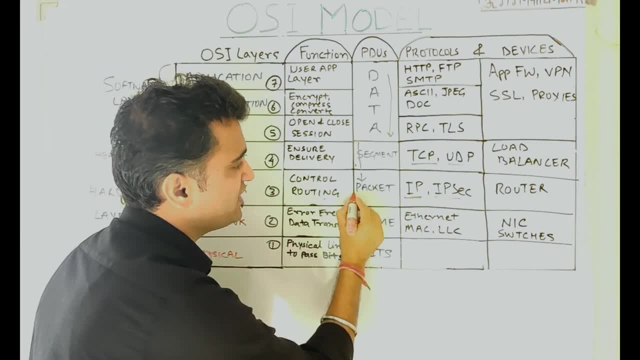 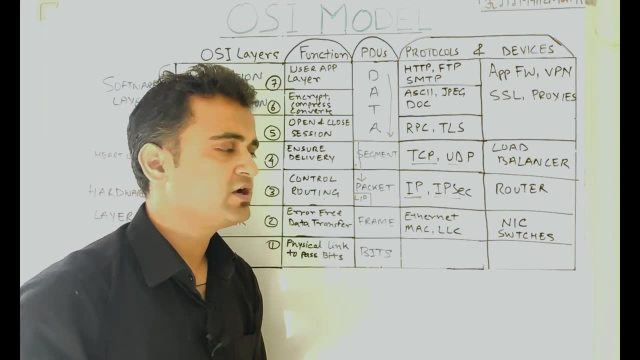 And that is where your protocol, IP protocol, comes in. So what you can add here? You can add the logical IP, Logical IP, Logical IP of the destination where you want to send this packet to. So this logical IP address could be added in this particular packet. 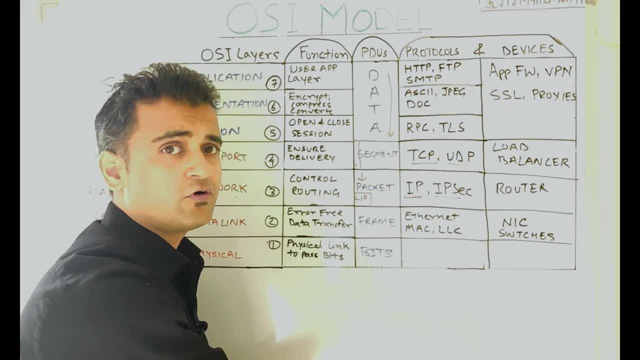 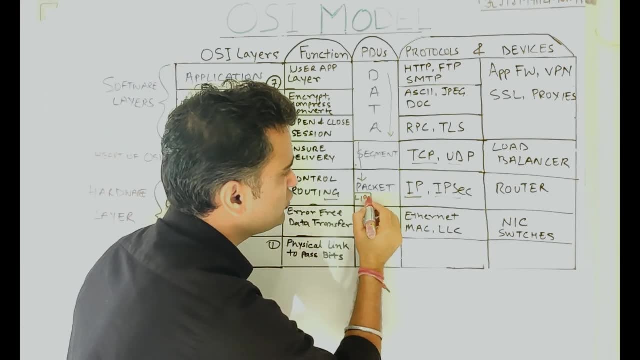 And the most importantly, I have not touched the devices for now. we will touch it at the end, But this is where your routers comes into picture. So, what you will do, your segment comes down. Now it has become a packet, because now you have the whole segment and with that we have 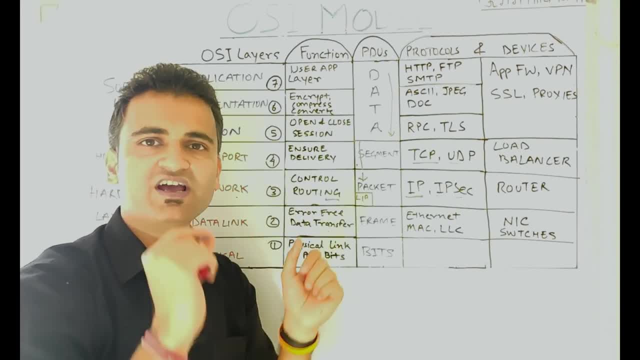 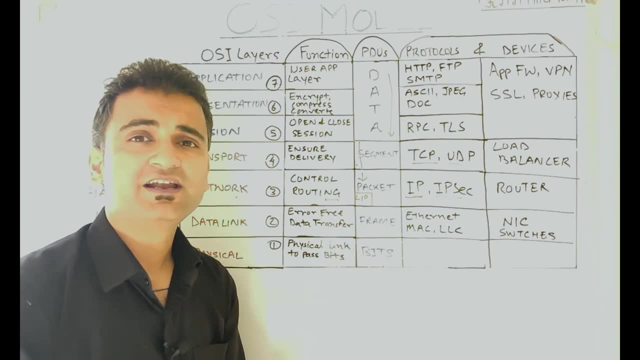 an additional network header, Which has become a packet Okay, Which has the logical IP address of the source and the destination, Moving down from the network to the data link layer. at the data link layer you have to ensure that the message goes to the destination error free and in perfect sequence. 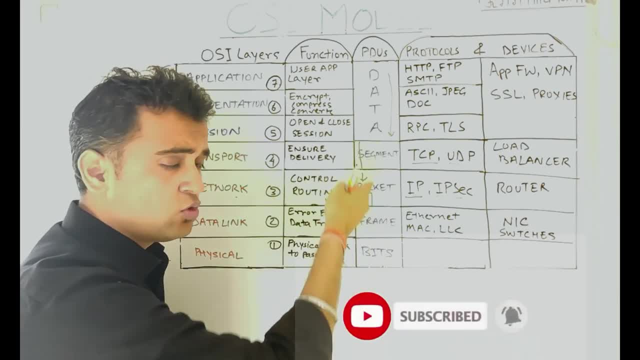 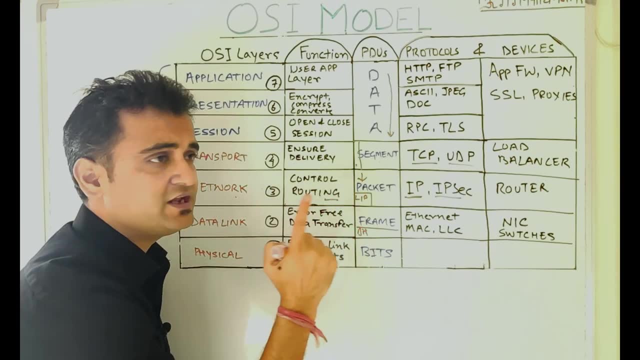 So that's why all the packets which are made here goes down, and then these are further divided into frames. So what it does? it adds a data header. So now you have three headers. You had segment, Okay, You had transport header. 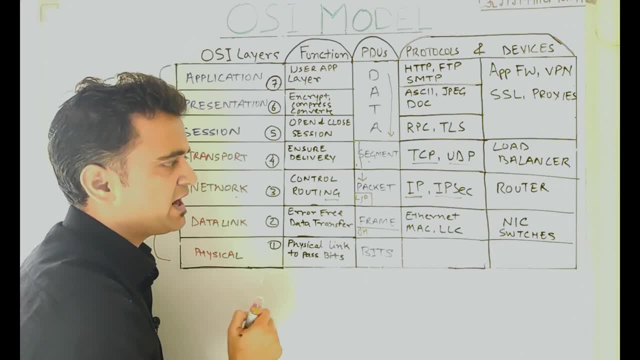 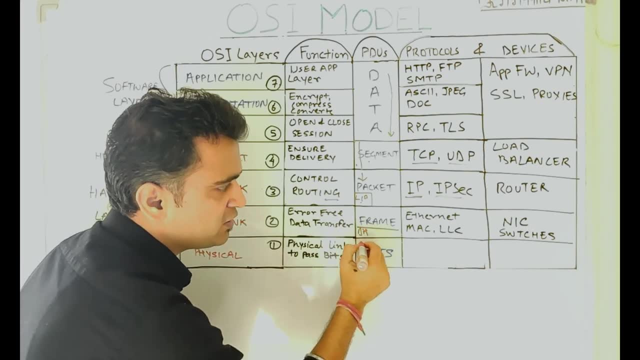 Then, in that you also added your network header, which made it a packet, Then you added your- you know- data link header, Then now it has become a frame. So in this particular frame, what you will do, you will actually have the Mac address. 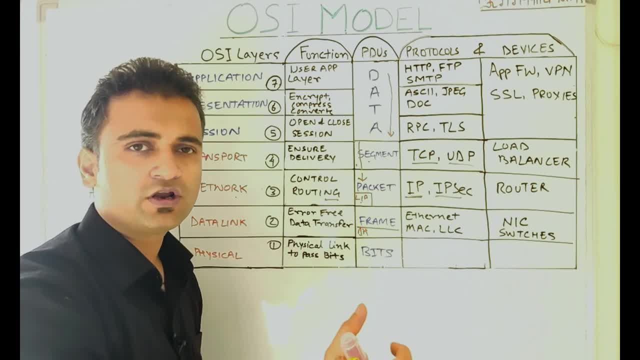 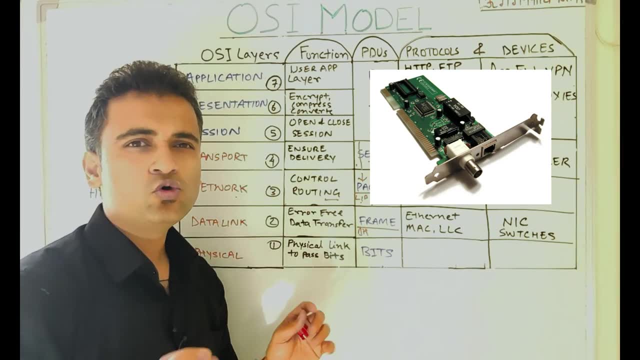 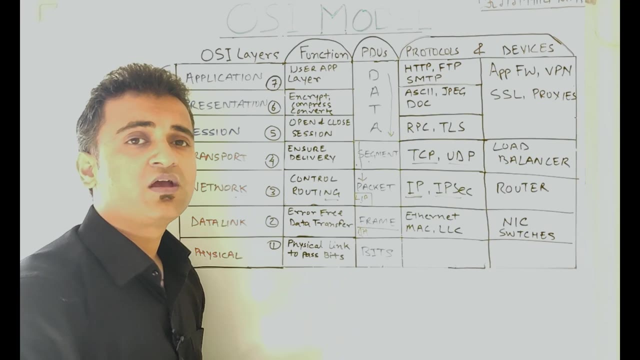 the Mac address of the device where you are sending this particular information and how you get it. So suppose in your laptops you have the NIC card, So your Mac address is universally unique. No two devices can have same Mac address, So that's why you will append that particular data in this particular- you know- frame and 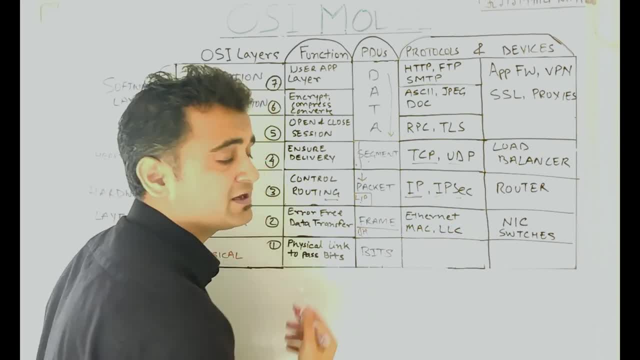 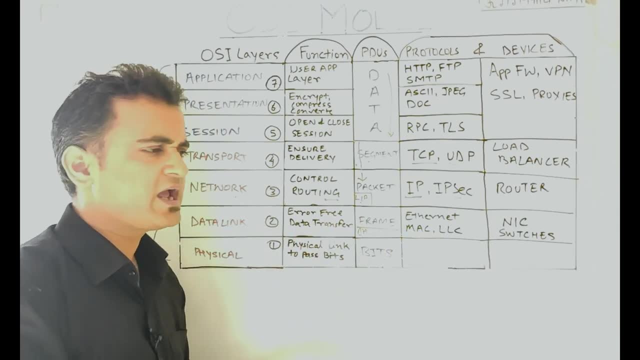 then it will send, send it, And the protocol which we use here is ethernet, And this data link has two main, you know, functionalities like Mac and LLC. These are subtypes of the data link, So this is media access control. 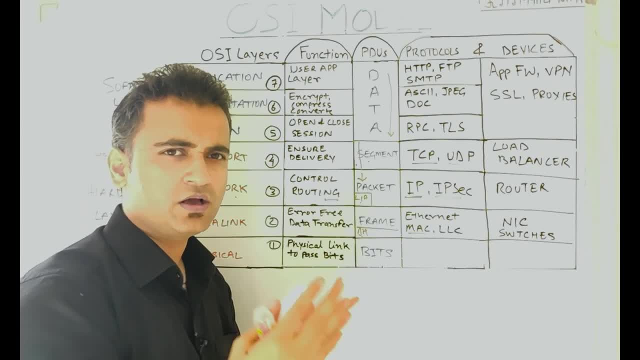 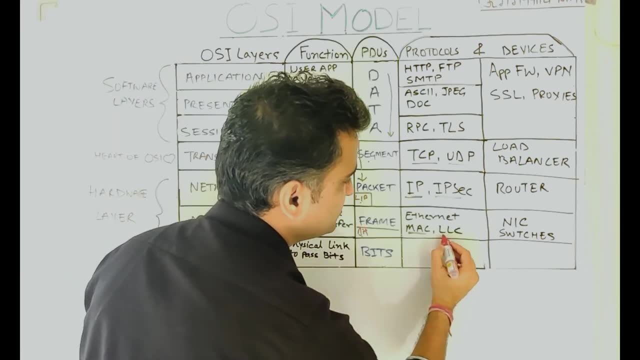 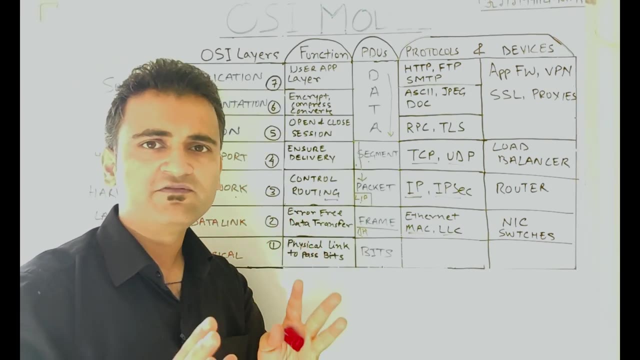 So which actually makes sure that the media goes in perfect sequence and you know it goes through, which is the functioning of media access control. Okay, And this is logical link. So this particular LLC functionality is to make sure that the delivery is error-free. 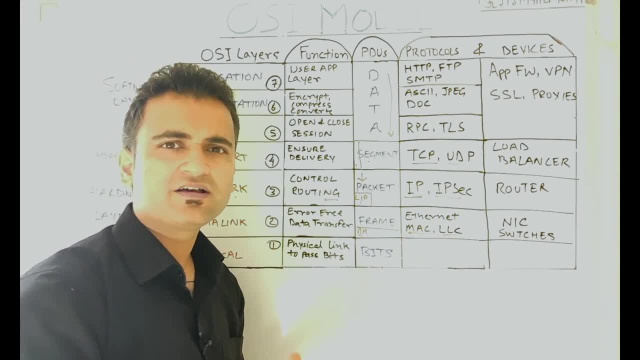 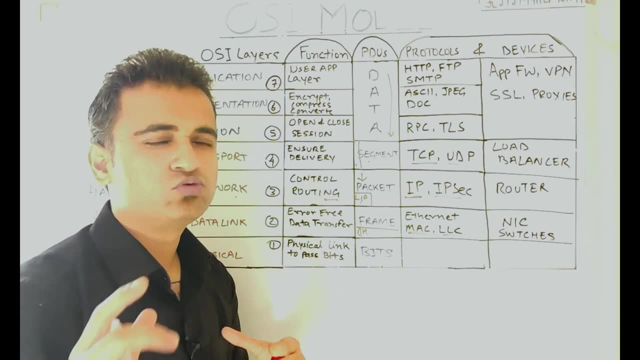 and that is the functionality of LLC. So there is a concept called as frame check sequence. So in that you need to understand that, whether the frames are going in the correct sequence or not. but those are very you know. next level of details: 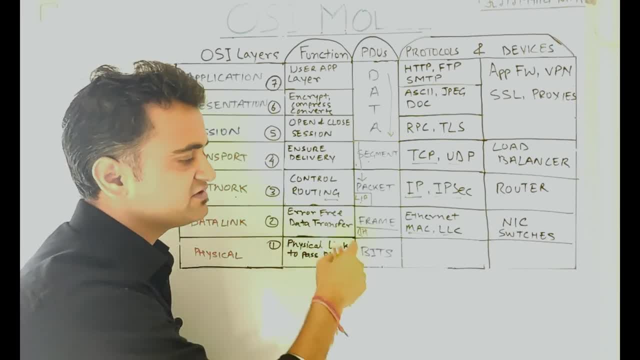 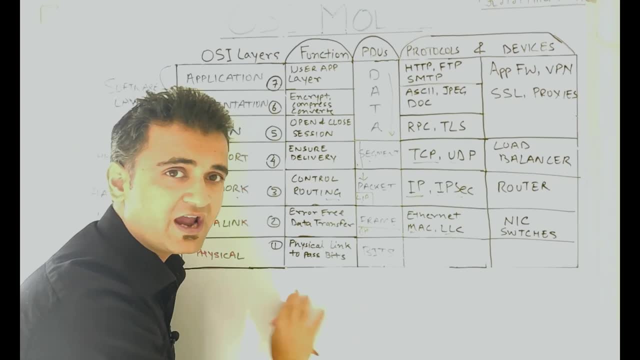 But to understand, a data link layer has your Mac address. that Mac address attaches to make it a frame. And then this particular frame finally goes to the physical layer, where your cadet, your ground worker. this is, this is where your actual fiber optic cables or your network, 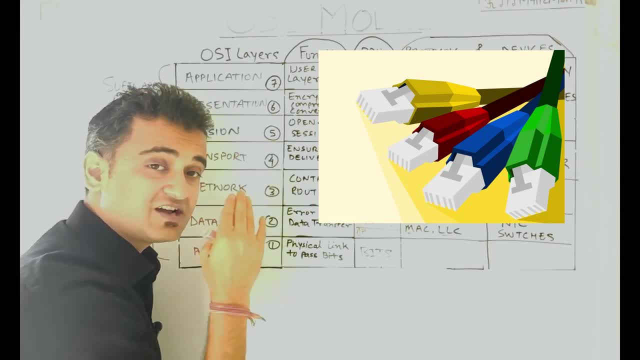 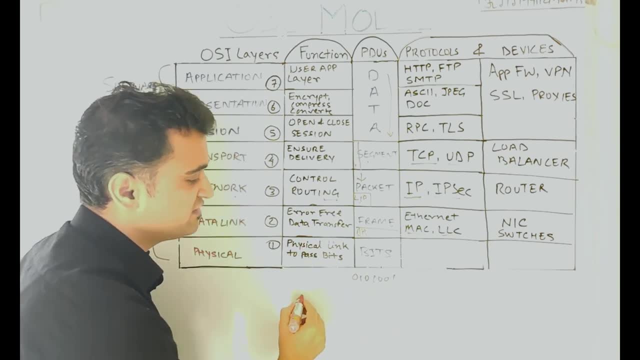 cables, RJ 45 cables- resides and converts this whole frame into bits. And what are bits? Bits are nothing but the binaries, and these binaries goes through electrical signals. Okay, So basically all these binary bits are goes through, as you know, voltage, pulse. 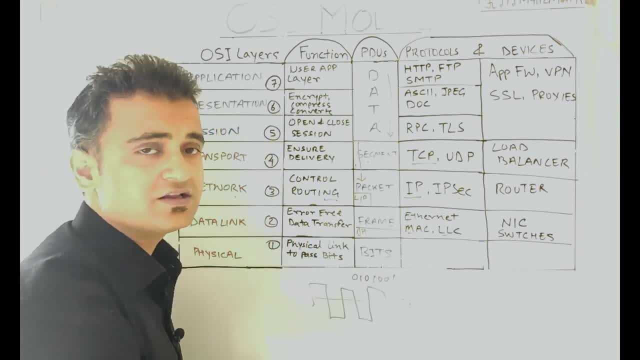 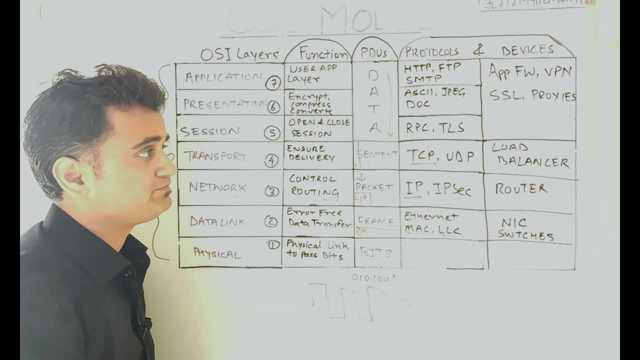 Okay, Through the network, Okay, So these are the- you know- seven layers and how the data is transferred. again, when it will be received, it will be received from bottom to up. And now, what are the devices which we use? now, when we understand the devices, we actually 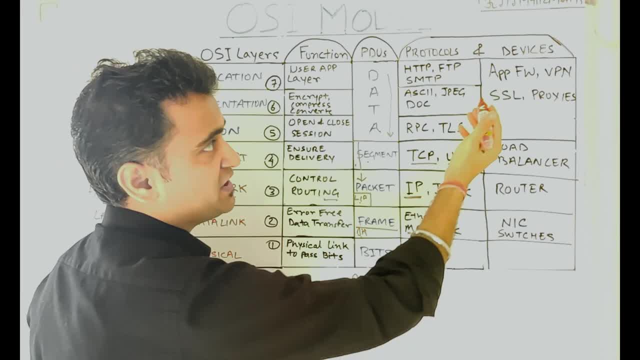 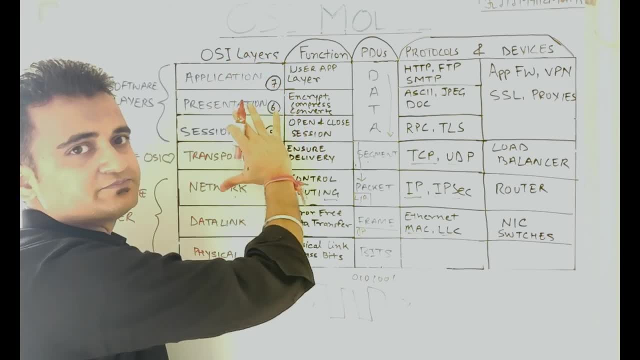 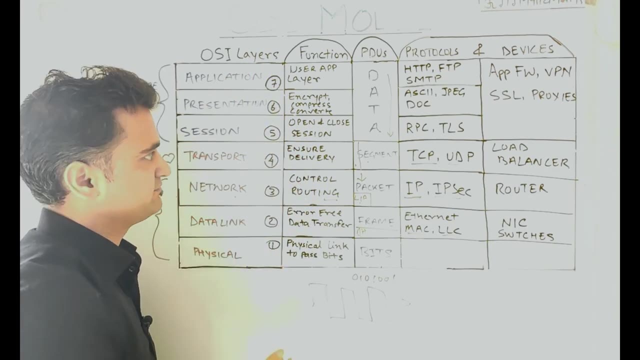 try to correlate it better. this whole model. So application firewalls, VPNs, SSL, proxies, all these kinds of concepts reside in your top three layer. Okay, These are the your top three layers, where these are. you know, These kinds of devices and methods resides at the transport layer. 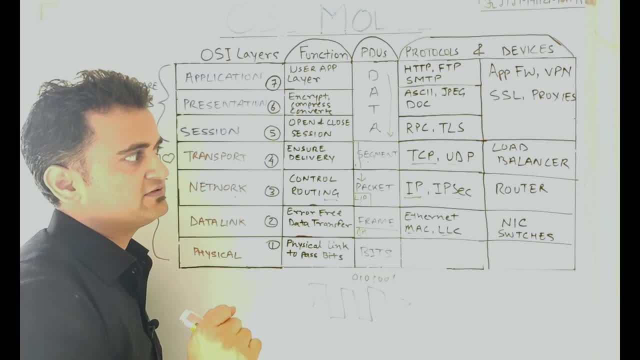 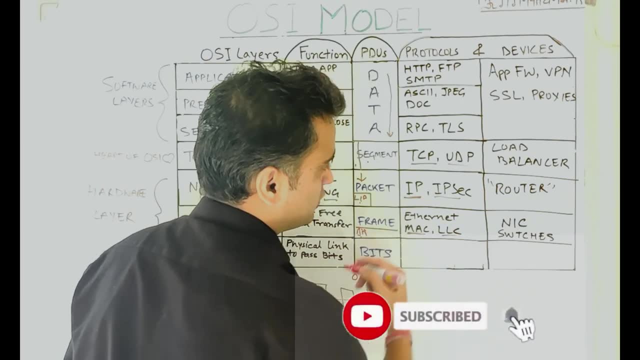 You have your load balancers. You might have seen the load balancers are working here, Okay At you know, at your network layer you have your all famous routers. Also, many people ask me in my previous video what are layer three switches? 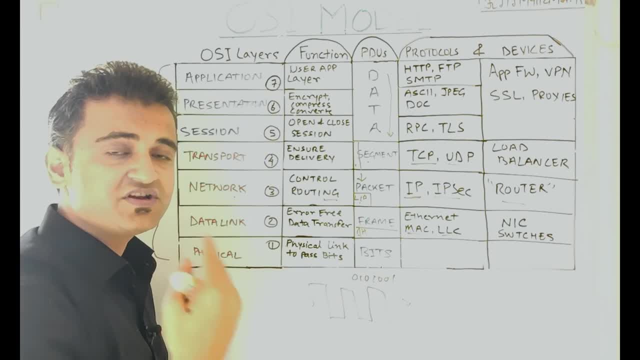 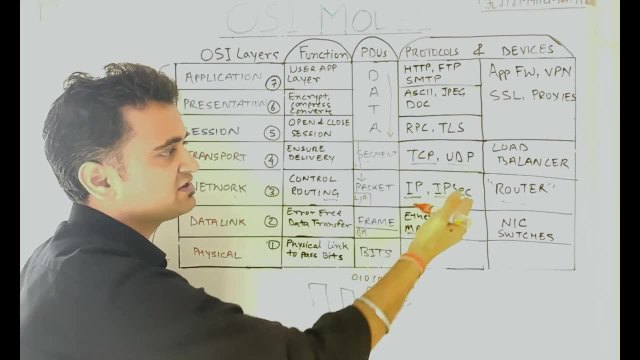 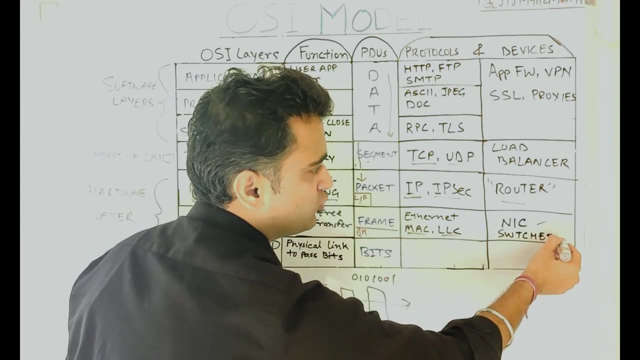 So layer three switches resides here and they have some additional functionalities which I've explained in that video, compared to what you know. You have your layer two switches, so layer three switches has more intelligence involved, in that In the data link layer you have your network interface cards and your layer two switches. 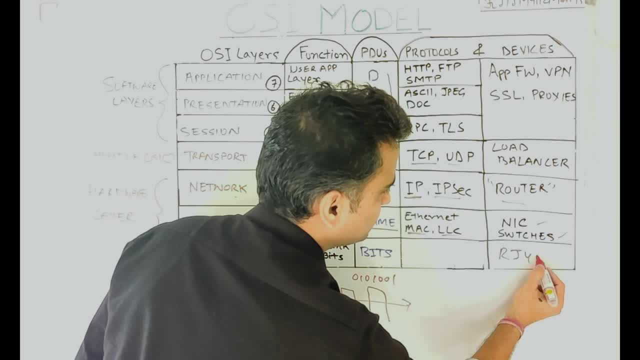 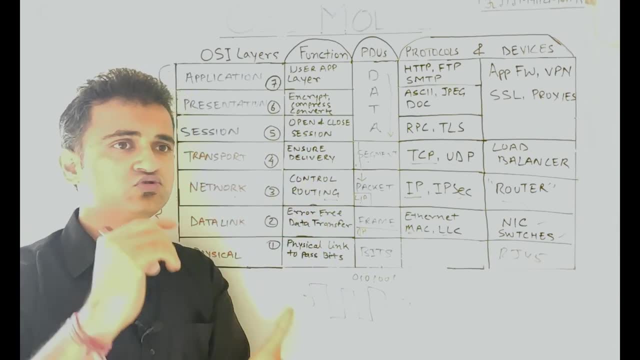 and in the physical layer you have your RJ45.. So, friends, as I said in the beginning, this is just a reference model of framework to fit our whole network flow into some sort of a framework and give us an idea that when we are talking about one specific network communication. 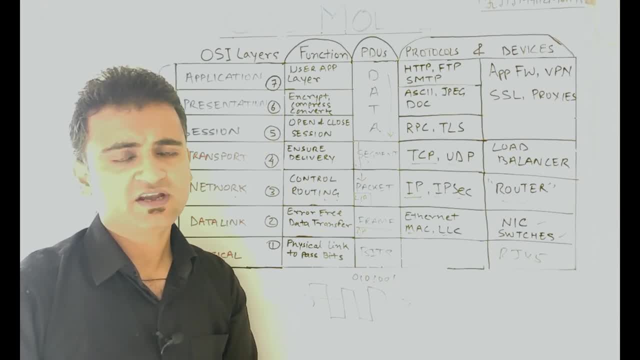 Exactly it is. you know it is fitting in. so suppose there is a network issue wherein you say that you know you are not able to access the web server and you are getting a firewall error. so you now know that if it is a firewall error, it could be residing somewhere you know in your top three layer, because 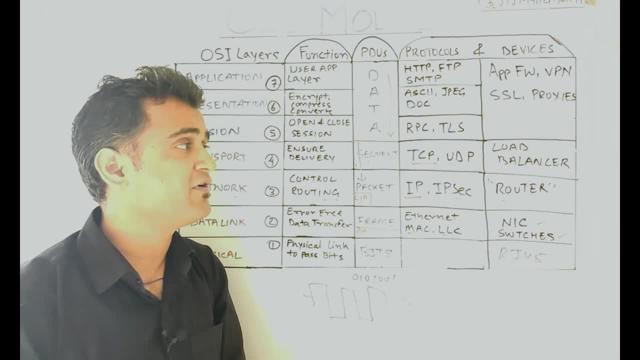 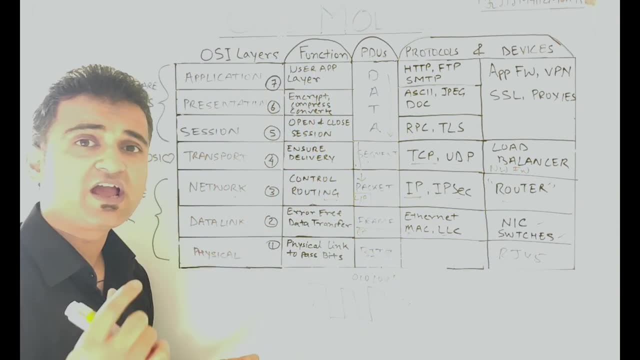 your application firewall resides here, but there is another network firewall. okay, so those network firewall. so I have not added it here, but network firewall resides here. so it can be that your application firewall is bypassed, but then there could be some issue with the network firewall. so now you can understand how you can, you know, help, take a reference like this and try to. 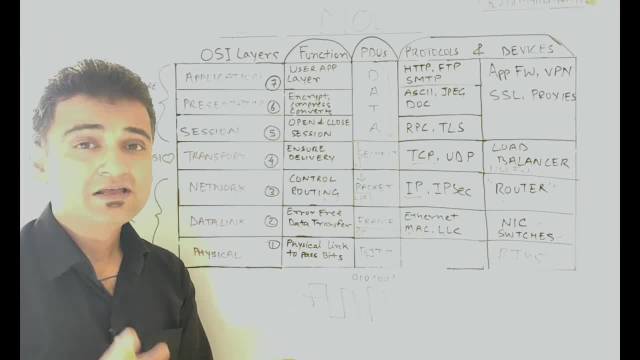 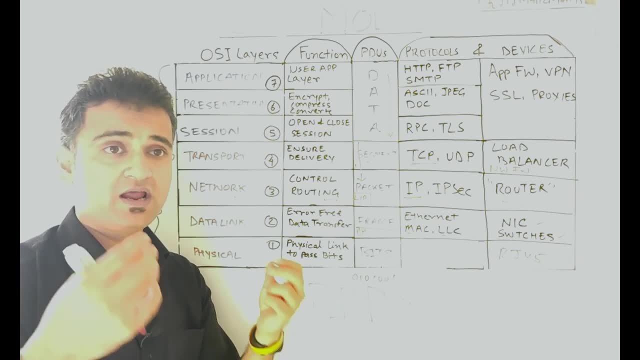 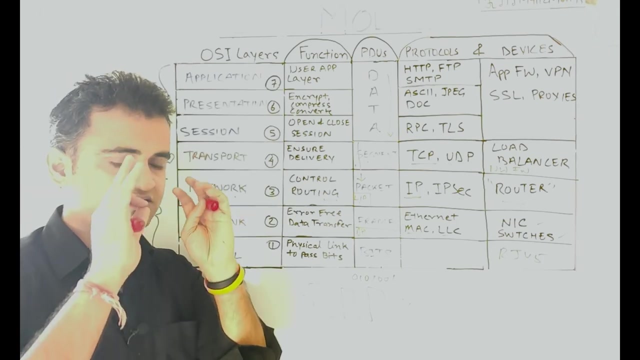 troubleshoot networking issues. but, as I said, this is a theoretical model. there is a much more practical model, which is a TCP, IP model, which is more prevalent and very practically used, wherein some of these layers are have been merged together, and this I will quickly tell you so that you know, you can understand that. 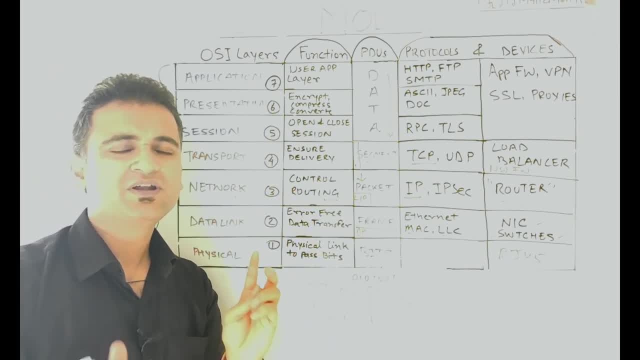 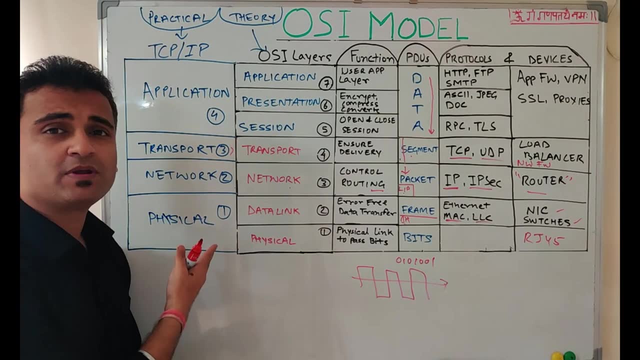 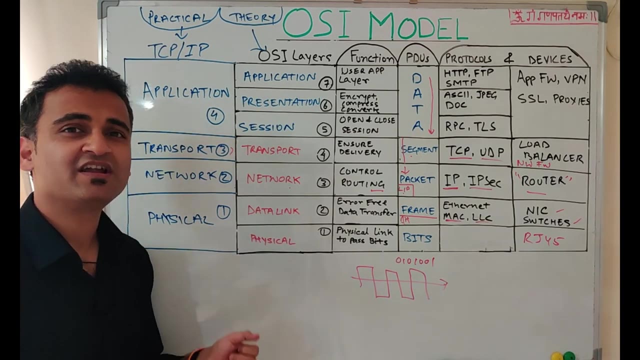 how OSI model and TCPI model are pretty much the same, but with with a slight twist, so let me draw that out for you. so, friends, this is the TCP IP model, slightly different from an OSI model. instead of having seven layers, this has only four layers. some layers have been merged. it is to give a more. 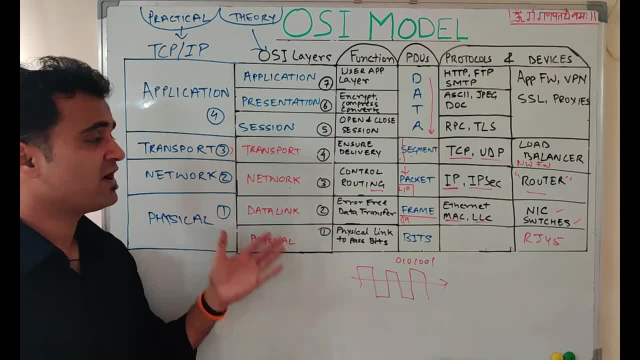 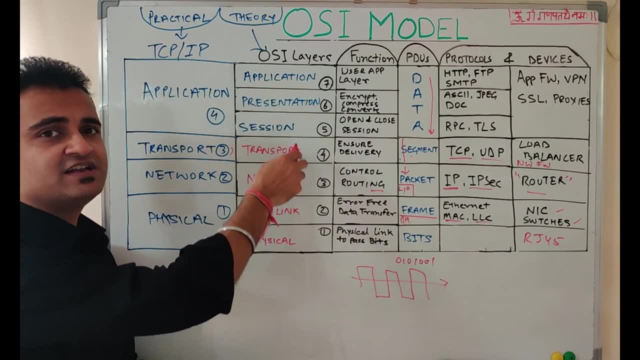 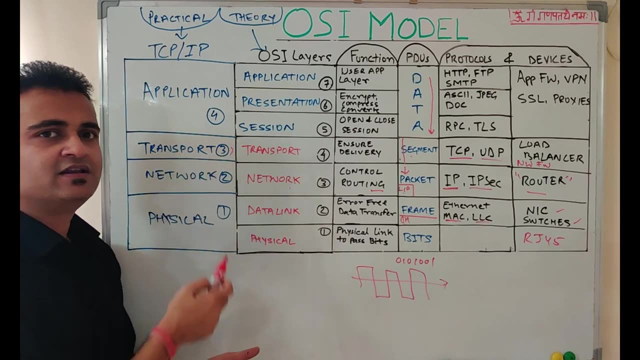 practical approach to this whole OSI model. so instead of having seven layers now we have four layers. so at the top the three layers have been merged. so application, presentation and session layers are now merged into one layer, which is the topmost fourth layer, which is the application layer, transport layer is at layer three. network layer is at layer two. so 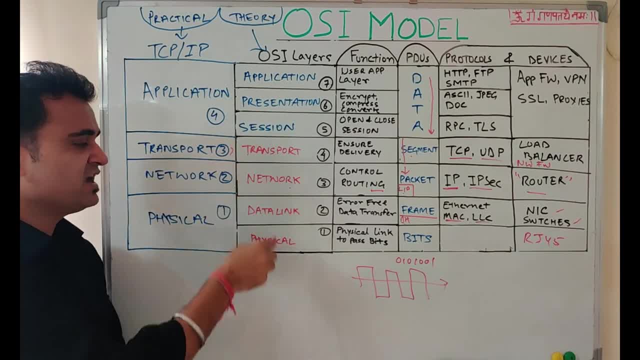 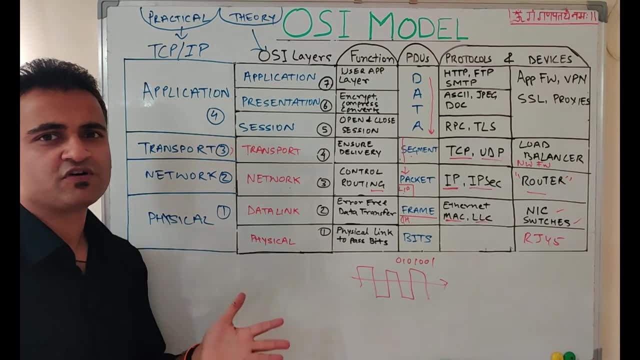 these two layers are intact, as as per the OSI model, and again the bottom two layer, the data link and the physical layers, have been merged into one common physical layer. but from the functionality standpoint both models are almost similar and gives you a reference point to understand how a network communication occurs. but 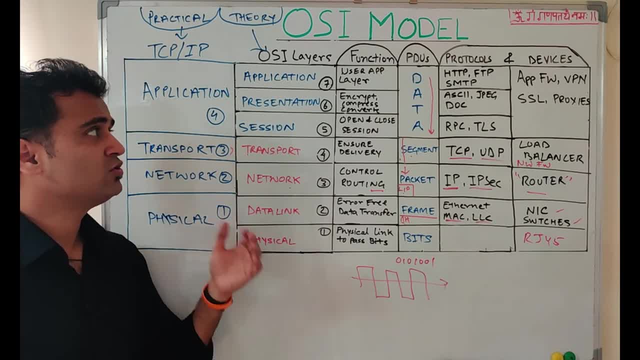 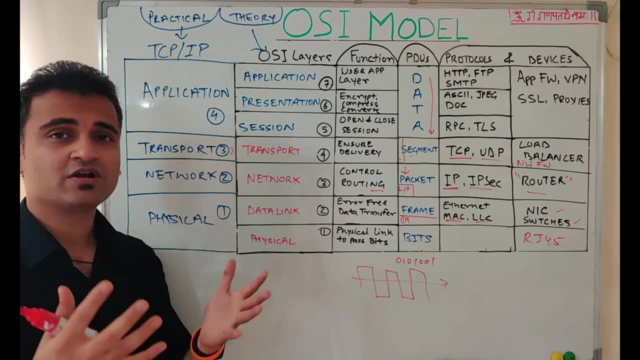 again, as I said, while designing, you need to be flexible. don't take it by the book, don't take it, you know. just take it as a reference point. don't make it too rigid. it is just for your understanding. so, if there would, there is always room to swap some of the functionalities here and